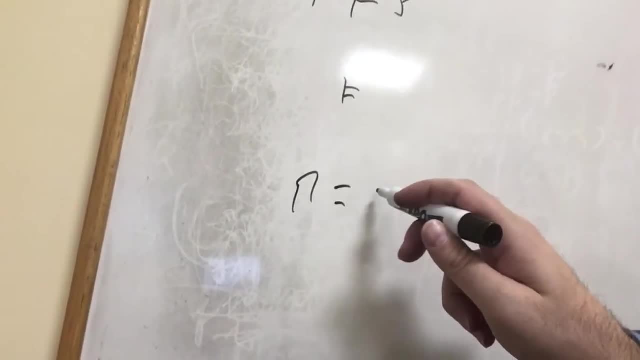 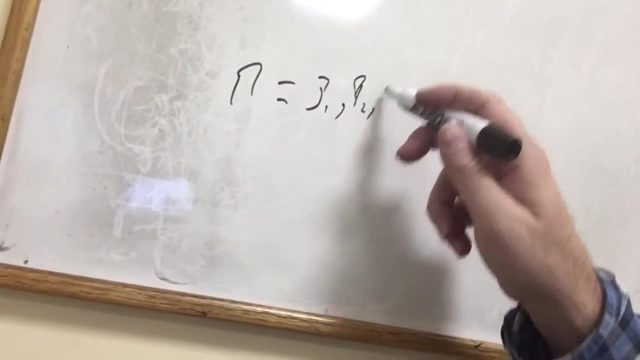 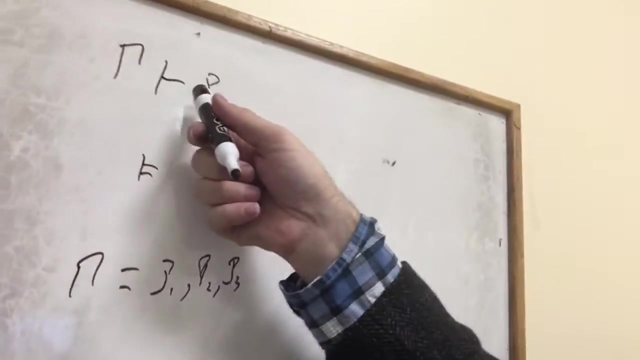 to stand for something. This set of premises, can it mean that some set of premises, so the premises may be p1,, p2,, p3, etc. So these can mean whatever. So, for instance, in a typical case, this might be modus. 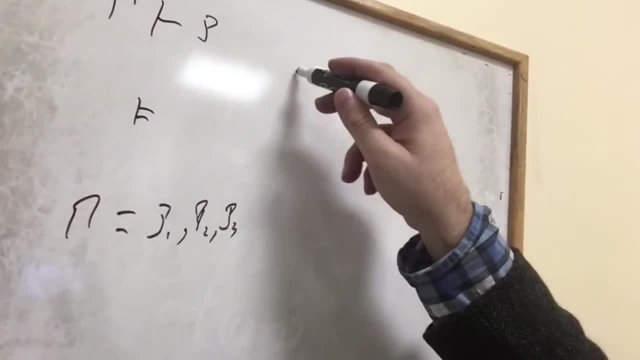 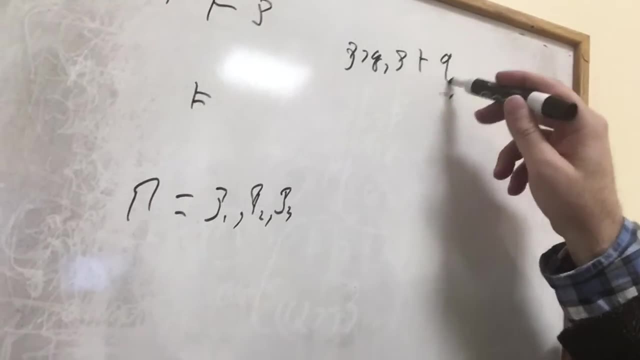 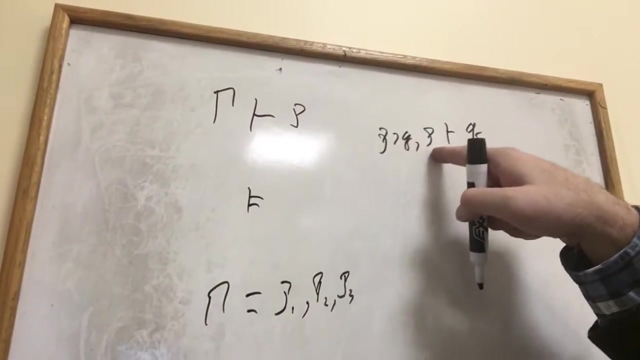 ponens. so from the set p, horseshoe q to p we can infer that q is the set. So gamma is an ingredient that turns out to be a set of premises. from a premise to a set of premises case here would be P, horseshoe Q and P, and sometimes people write that as the 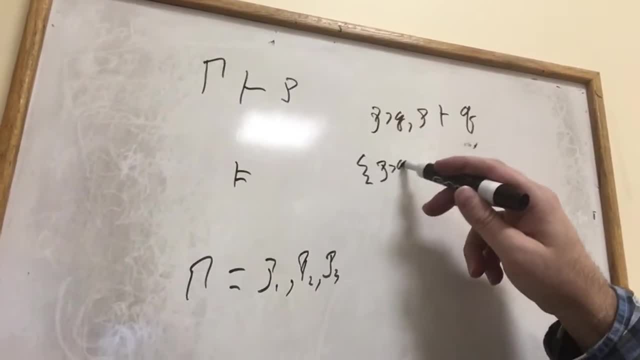 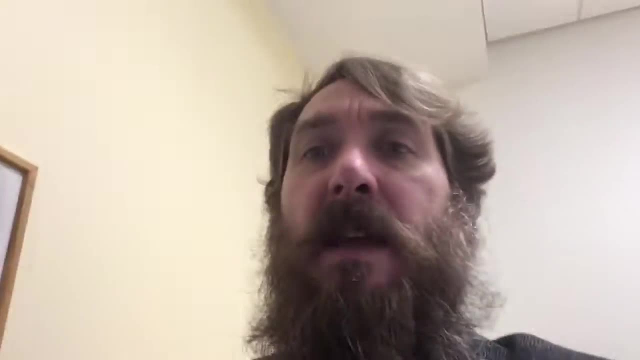 union of those things. so we would say that the union of P, horseshoe, Q and P. okay, so that's in the sort of language of set theory and we're not going to worry too much about that. but basically the idea here tells you that if you have 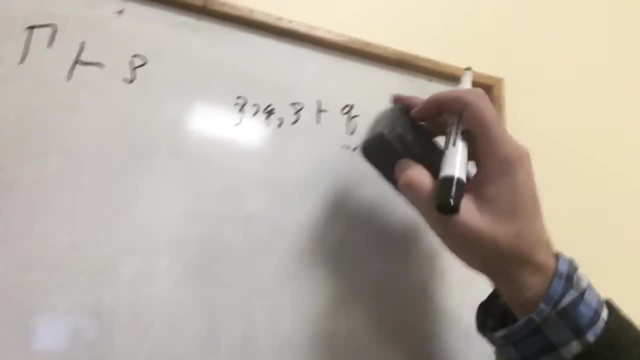 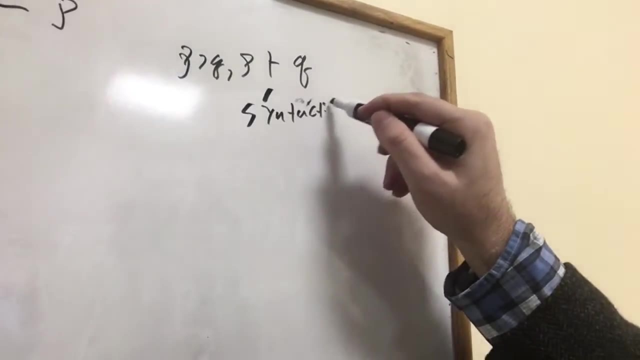 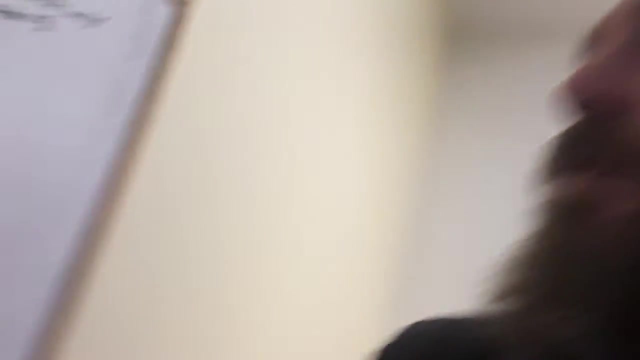 P, horseshoe Q, then that syntactically entails that Q and what this turnstile means syntactically entails what that means is that there is a proof starting from P, horseshoe Q and P and getting to Q, and we know that there's a proof. 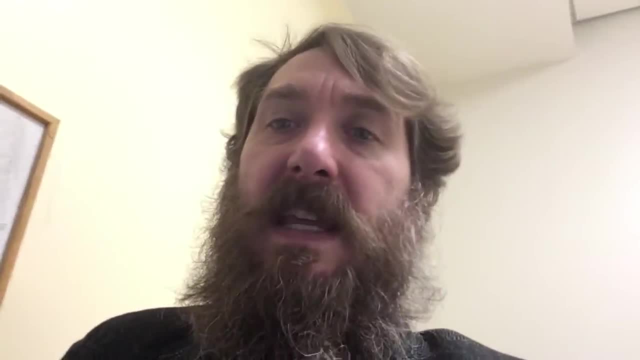 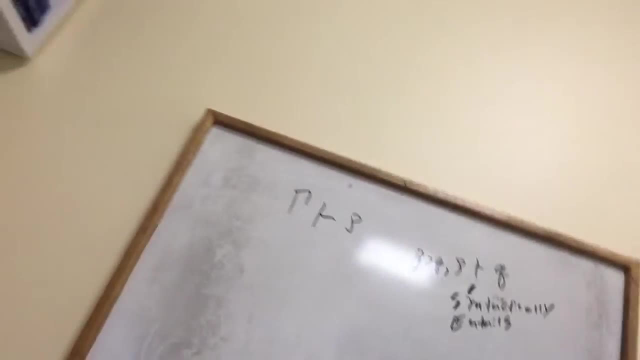 because that's just modus ponens and that's one of our basic rules. so we've taken that as kind of our primitive case here, and so we know that that's gonna hold, and so what we would like to be able to show is that everything. 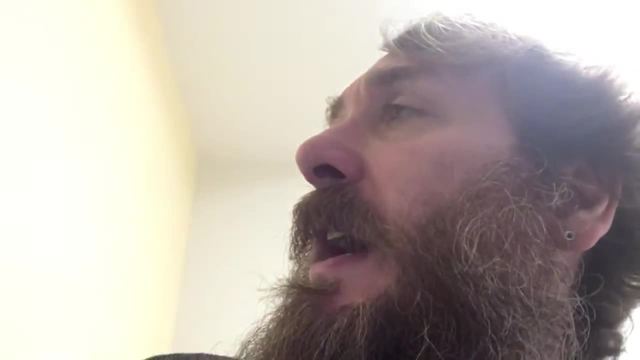 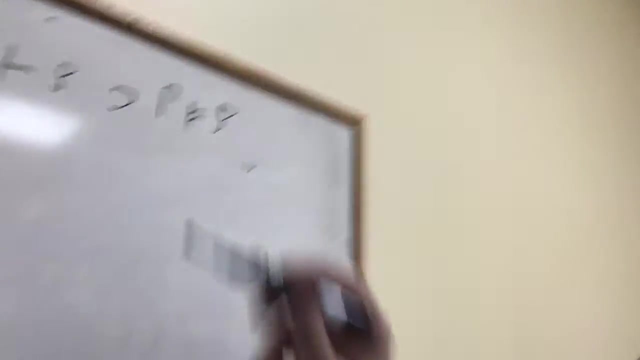 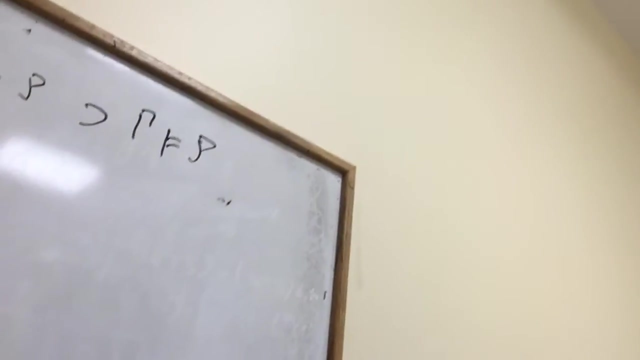 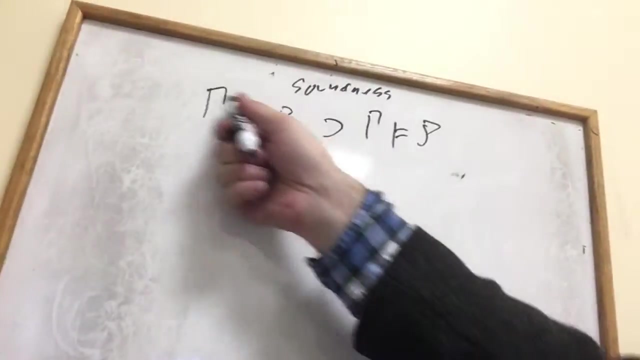 that we can prove. everything that we can prove is also going to be something that is syntactically entailed. so we want to be able to show that everything we can prove is syntactically entailed, and this property right here is called soundness. well, roughly, what it's saying is that all the things that we can prove, 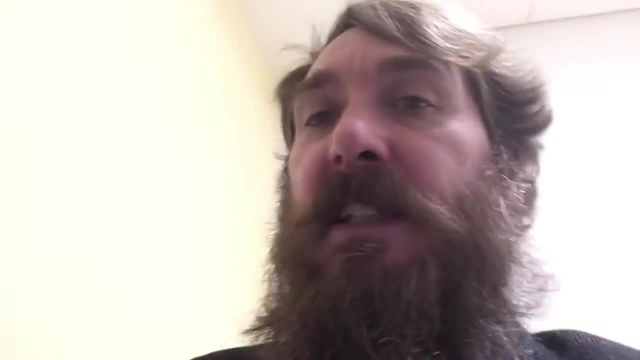 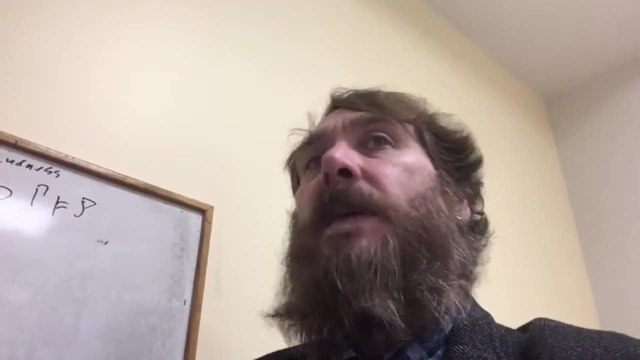 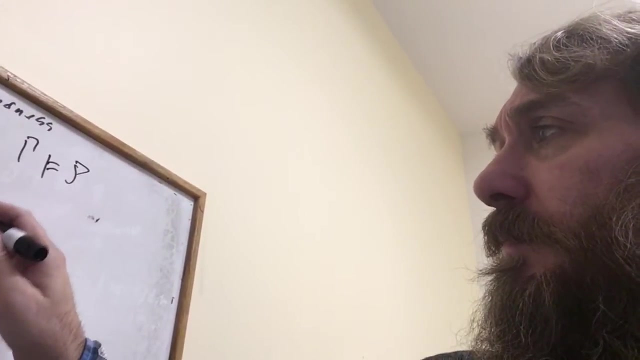 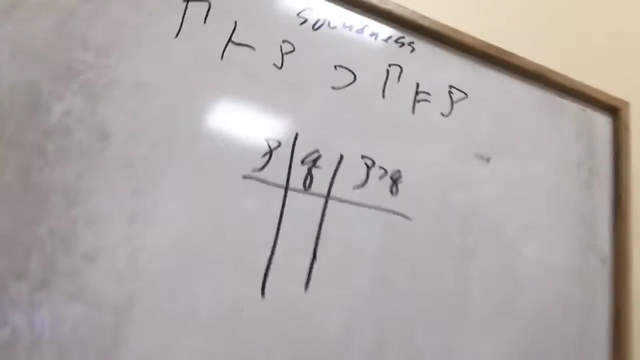 are things that we could semantically prove and syntactic entailment. remember, for us it is defined in terms of truth tables because this is a propositional logic and so, for instance, if we take modus ponens and we look at the truth table for that, and so the truth table for modus. 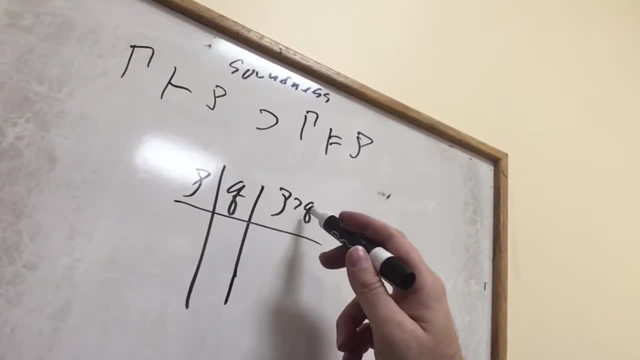 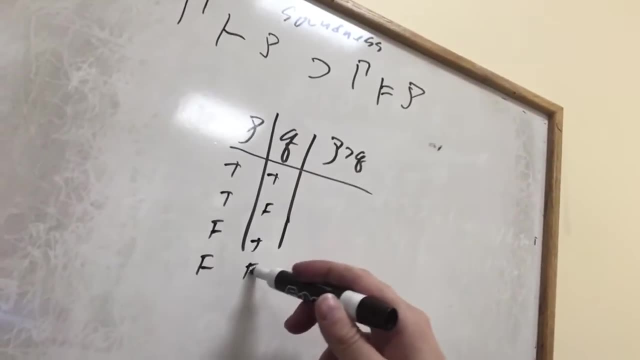 ponens, we know how to construct it. we have P and Q and P horseshoe Q, and so we fill in these values in the normal way that we have always filled them in as so, and then compute the horseshoe function in the way that we. 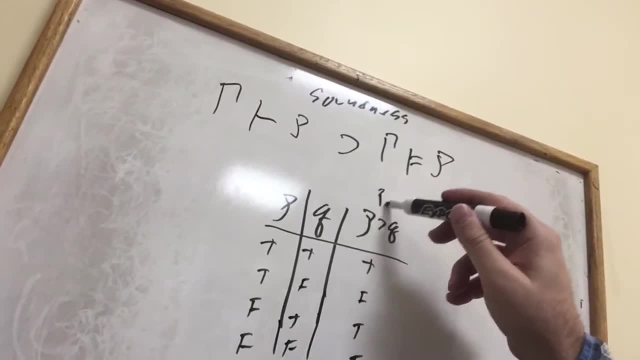 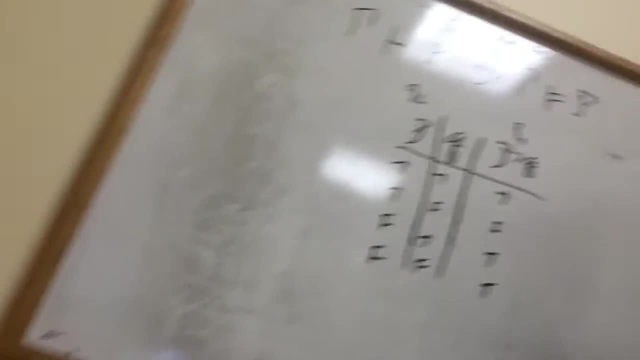 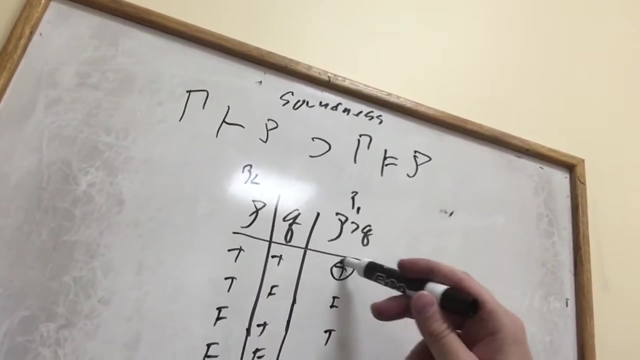 have always done. and so if this is our premise one here and this is our premise two here, sorry about that. and so if this is our premise one here and if this is our premise two here, then we can see that when premise one is true and when premise two is true, then Q is true and 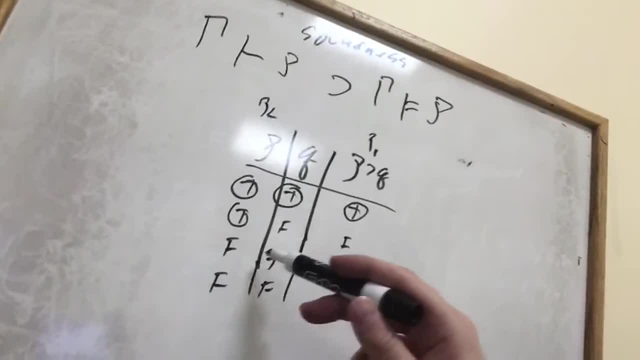 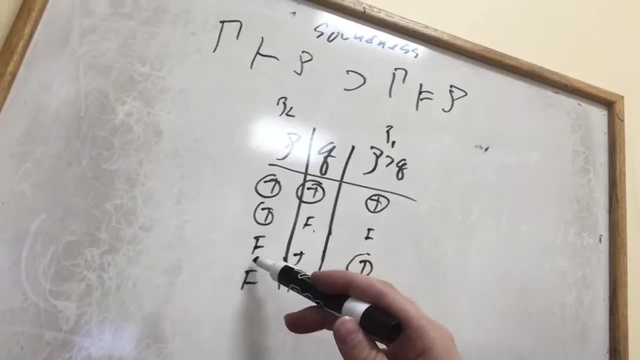 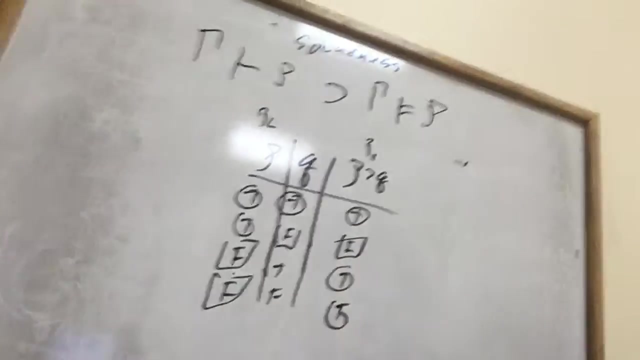 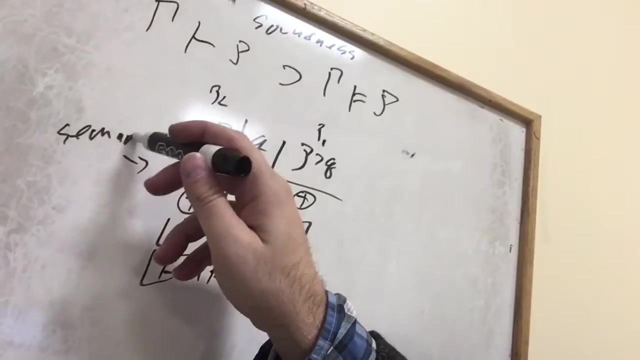 there were no other cases where they are both true. in all other three lines of our truth table there's at least one false thing. so Q- excuse me, P horseshoe, Q is false, P is false, or they're both false. so this right here indicates that there's a semantic entailment when one 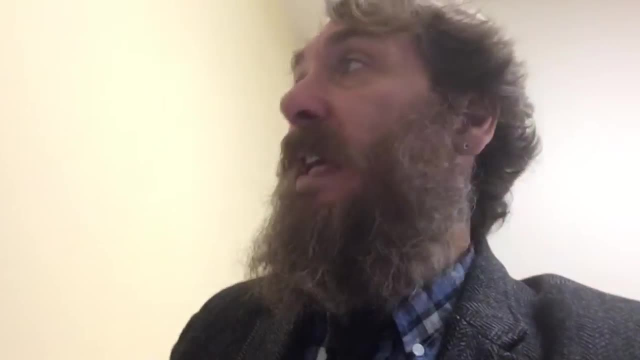 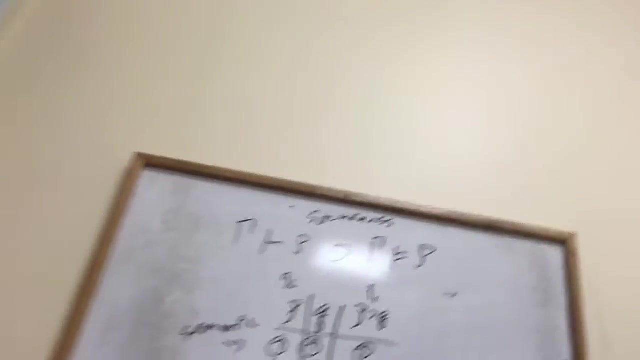 is true, that makes the other one true. so when P is true and P horseshoe Q is true, then Q has to be true. there's no other option. okay, so now soundness. if this were a more advanced class, we would try to prove soundness. 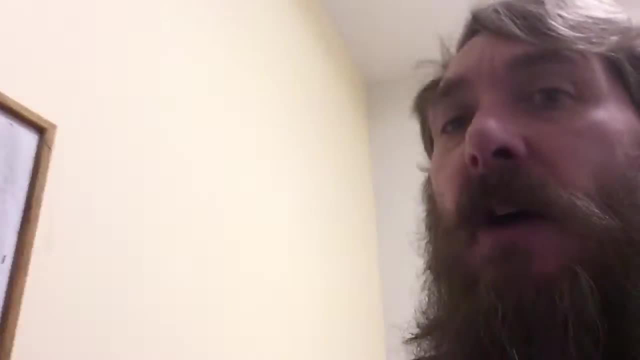 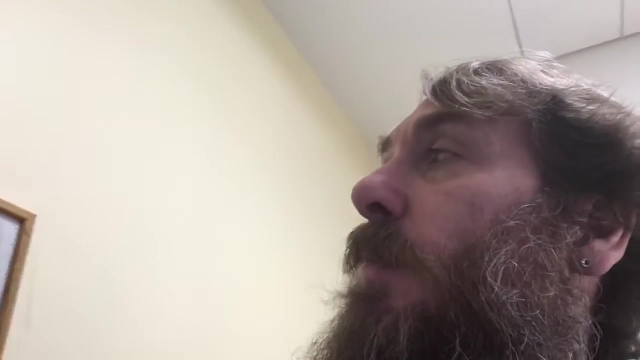 and we won't do that. but you can kind of see how it would go. it would be just taking all the rules that we have and showing that every time you apply one of the rules, you only get something that ends up in semantic entailment, and we 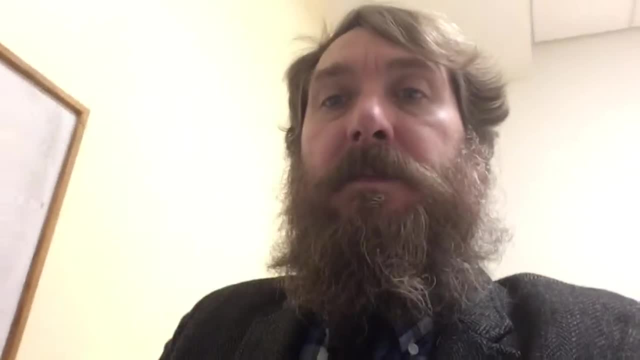 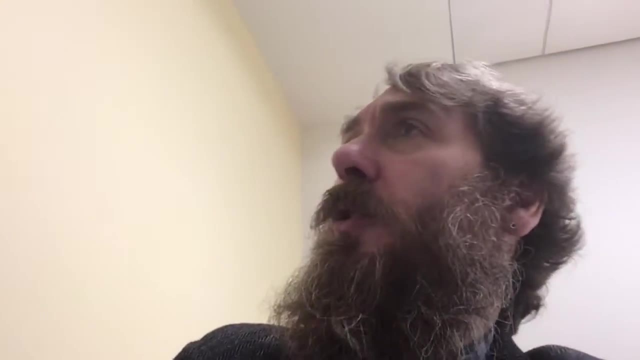 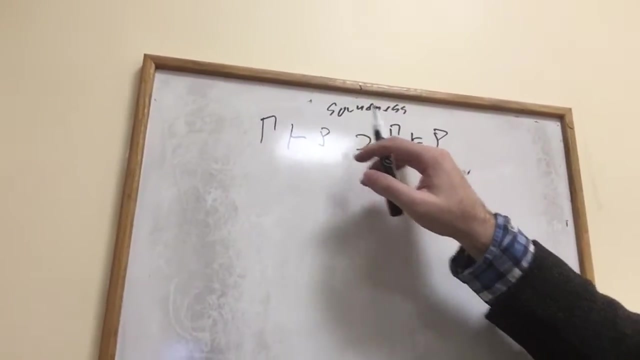 sort of just saw that with our looking very quickly at modus ponens. so in modus ponens there is a proof. we say that's a basic rule. we can use that rule to get to Q. and then when we look at the truth table, well, if the set over here is, 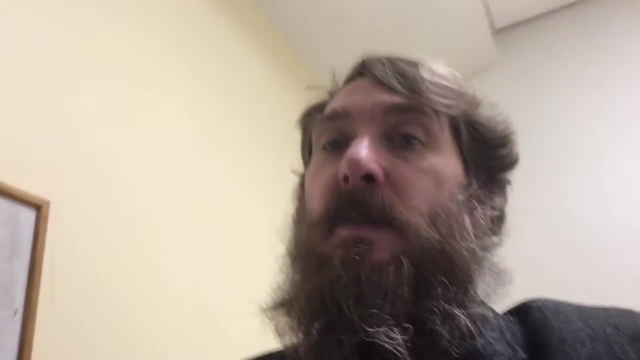 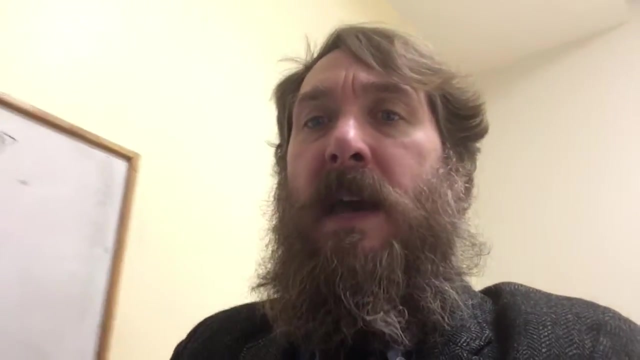 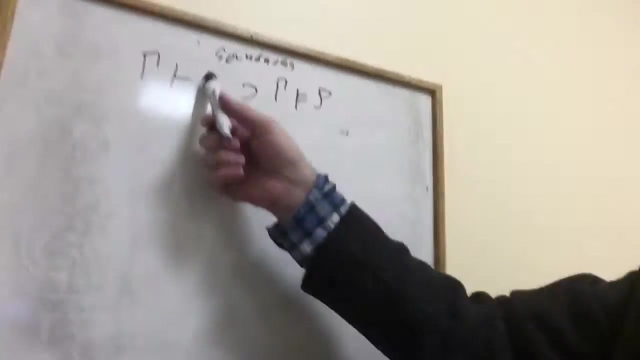 true, then Q is true, and so there is that semantic entailment, and so every use of that rule will guarantee that, and we can see that all the other rules that we have are also going to roughly function that same way, and we won't go through all of the 18 rules that we have, but in class we have been careful to. 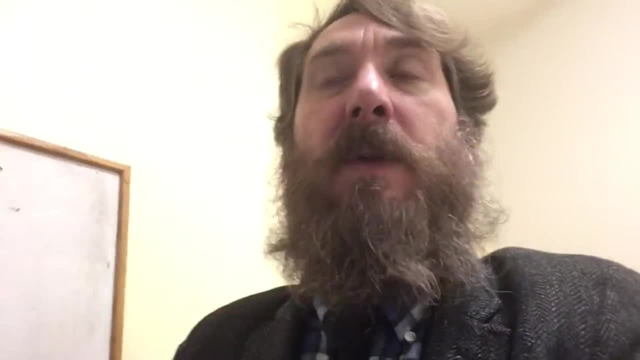 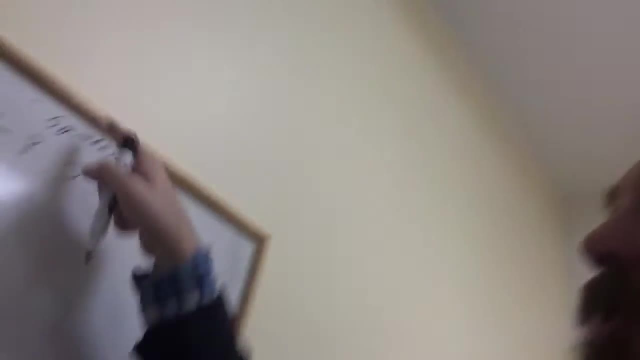 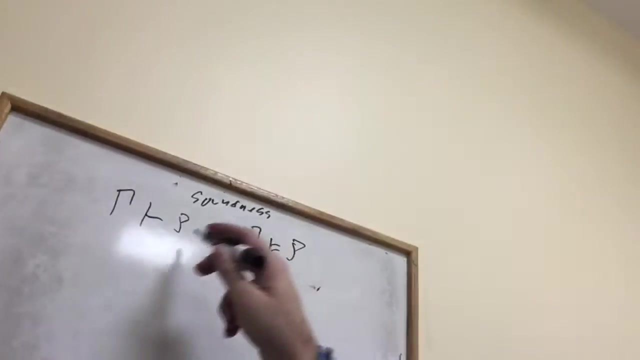 stop every now and again and to make sure that we understand how applying the rule at a syntactic level also make sure that we preserve truth. so soundness is relatively easy, although require some work to show the other property going in the other direction. which says that if a set of sentences semantically entails 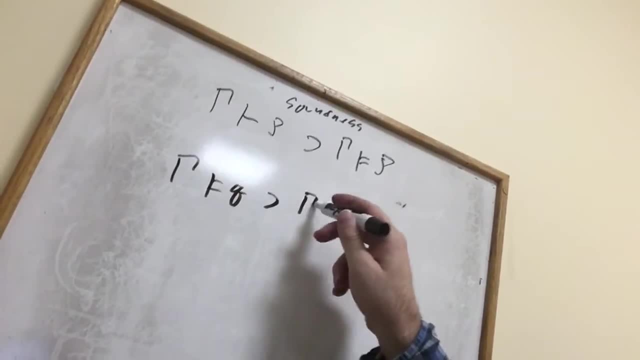 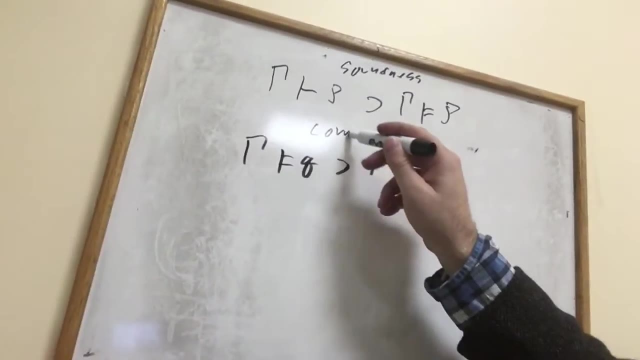 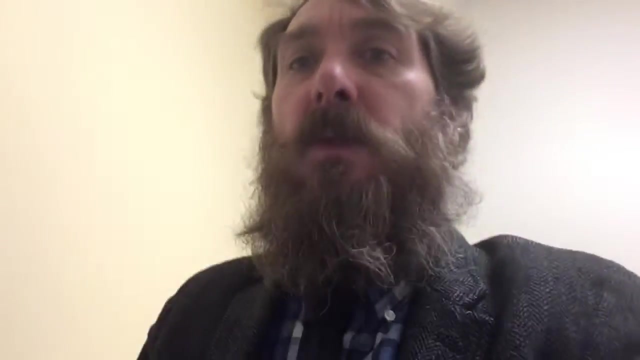 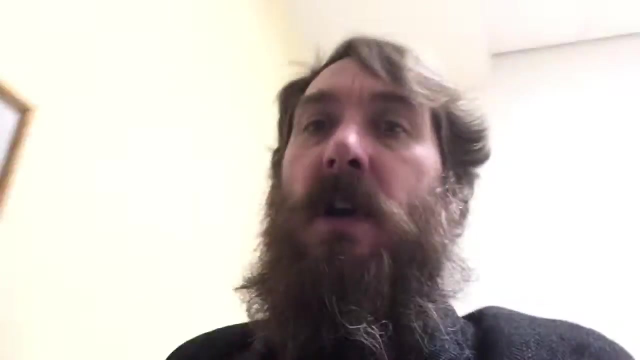 some other sentence, then that set of sentences syntactically entails that sentence and that's what's called completeness. so there are many different ways of using the word complete and we're not going to worry too much about the different ways that people have used them. but for us, 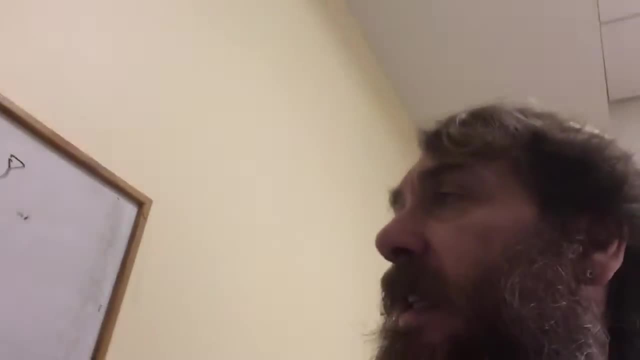 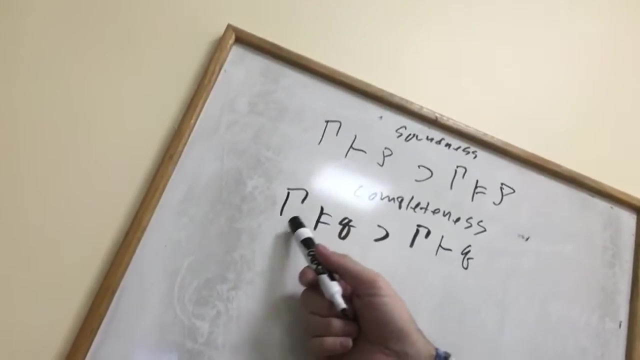 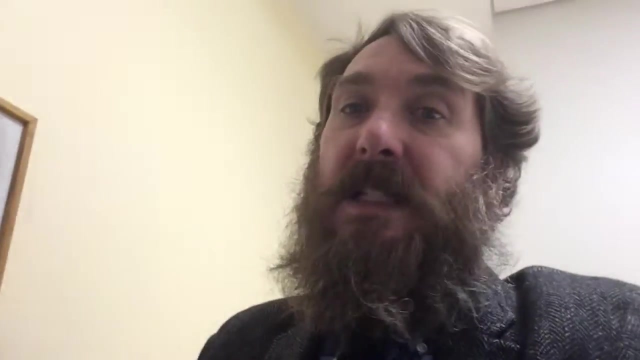 in the class that we've been dealing with. talking about completeness is talking about whether or not this property holds. so if something is a semantic consequence of some set of formula, then it's a syntactic consequence. so let's take the special case. we're not going to prove. 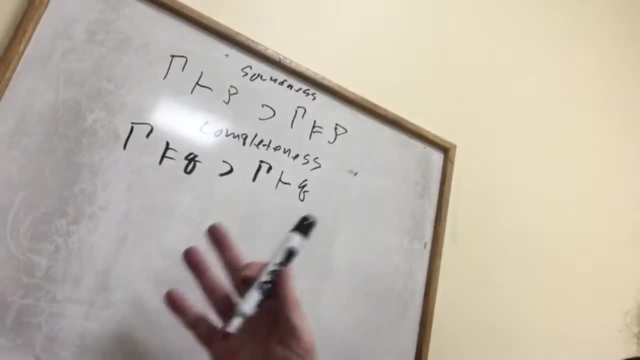 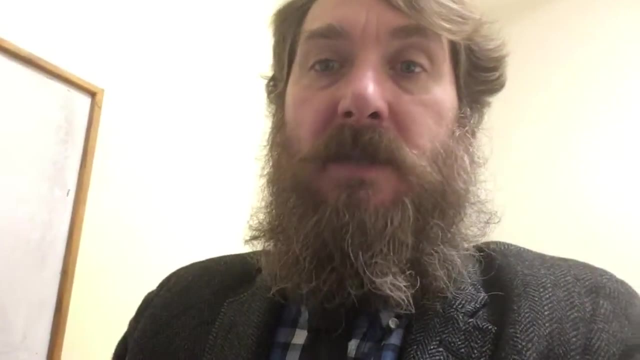 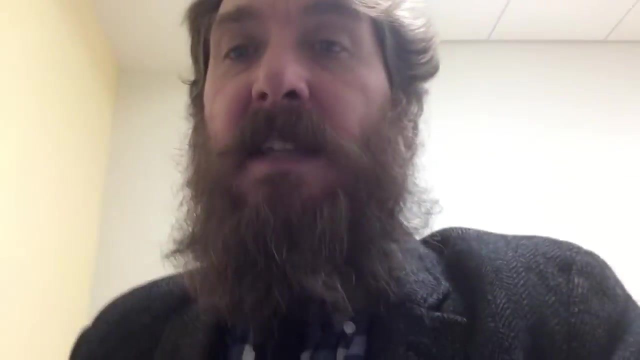 completeness, by the way, for propositional logic. but we can at least get some idea, get some distance towards seeing why it would be true for propositional logic. for the rest of the class, The basic idea is as follows. so let's take the limiting case where gamma is the 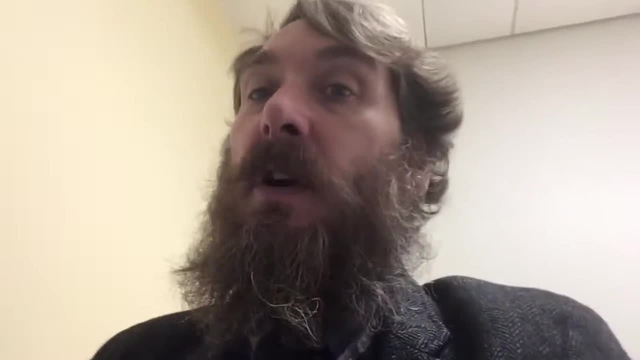 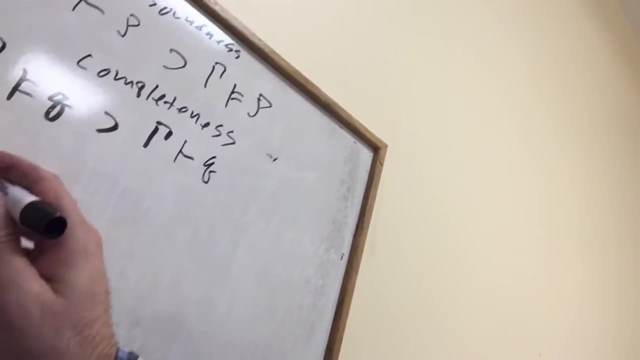 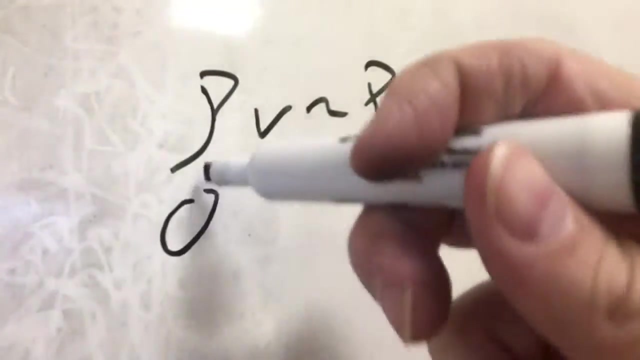 empty set and Q, therefore, is some kind of tautology. so let's pick a really simple tautology and let's pick P- wedge tilde P. so notice, I'm using kind of meta variables here, and in real life I would like to use Phi- wedge tilde Phi, or. 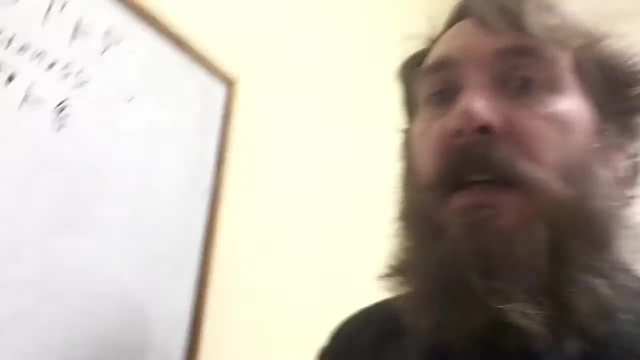 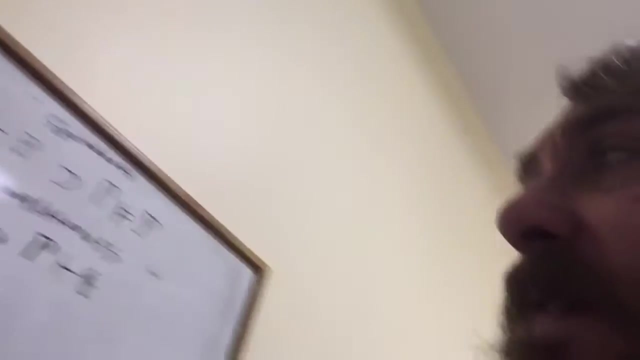 alpha or something like that. but because of the book we're using doesn't use those meta symbols, I'm using lowercase P's and Q's, even though that's kind of annoying, so we can look at this and the reason why it's nice to write it. 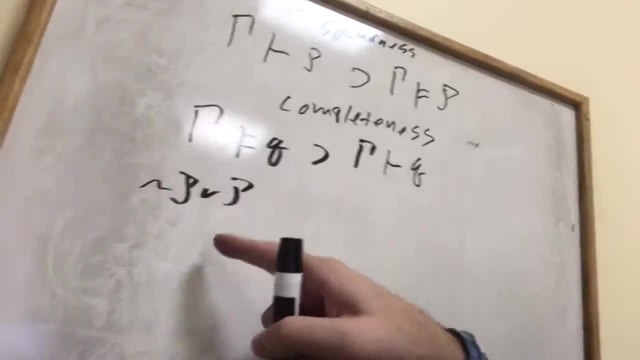 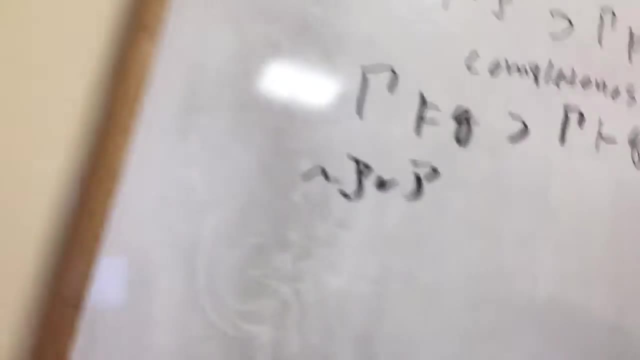 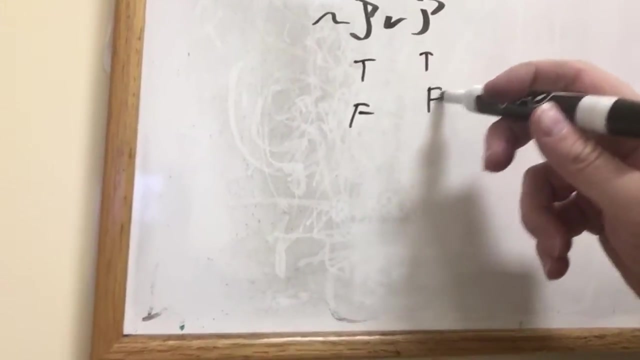 in meta variables is because now, P is any well-formed formula, and so any well-formed formula at all, no matter what, we can see that this is going to be a tautology here, and so if we just did the table in the normal way, there's only two terms here and the tilde sign reverses. 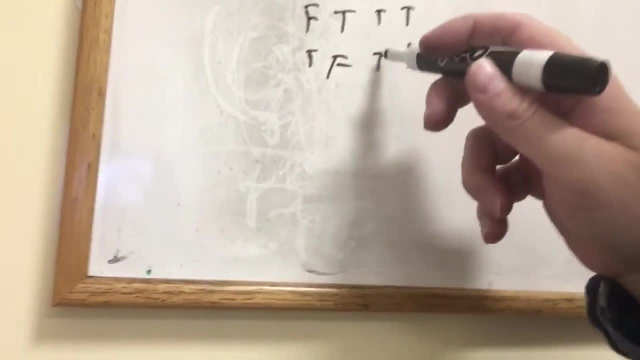 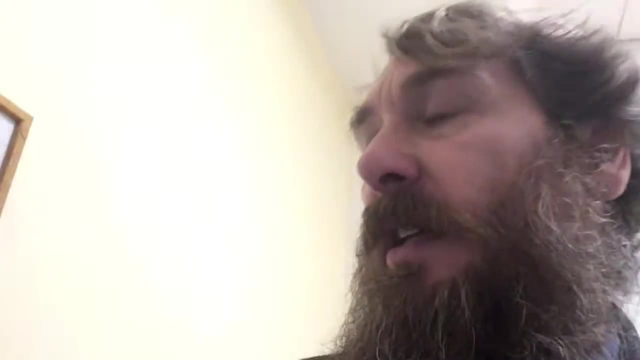 those truth values the wedge operator tells us. as long as one or the other is true, the whole thing is true, and so we can see that this is indeed a tautology. now that's interesting, because we can kind of look at this and then we can see: 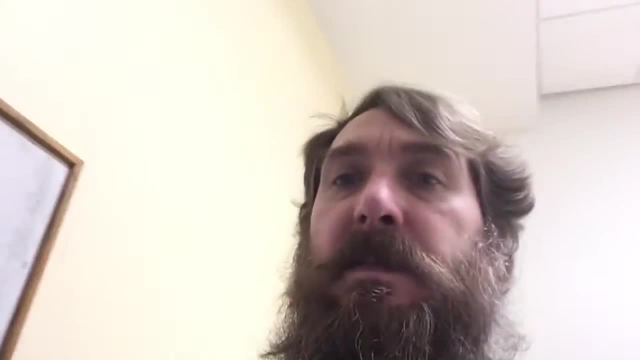 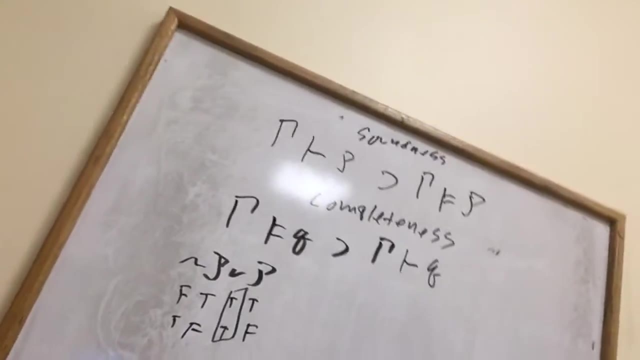 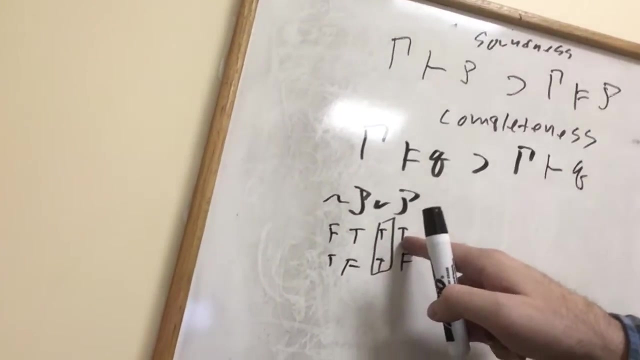 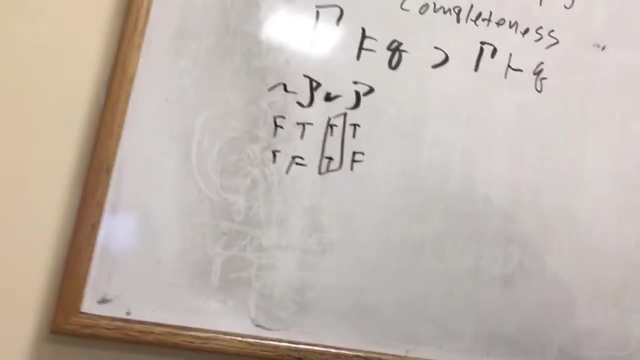 some interesting things. so using our definition, which we just introduced, of semantic entailment, we can see here that what this is telling us is if we look at the case where P is true, so that's the first line of this truth table right here- we look at the case that P is true and if we simply included 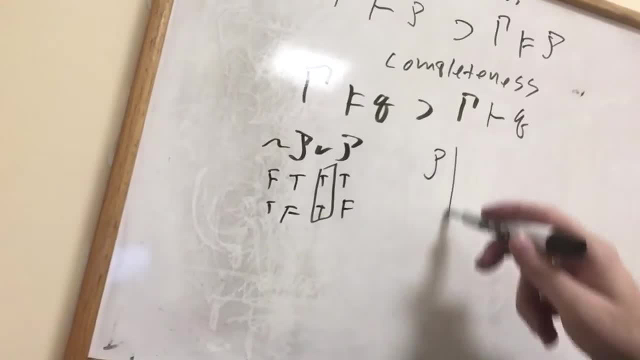 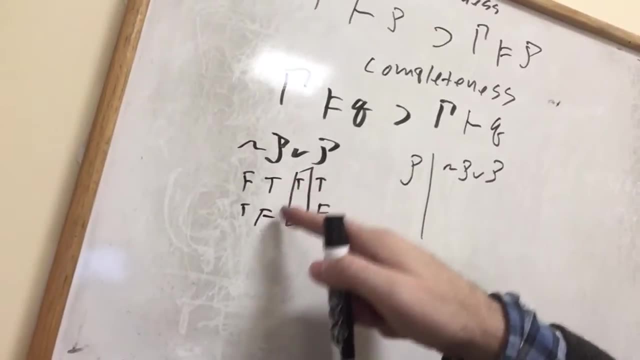 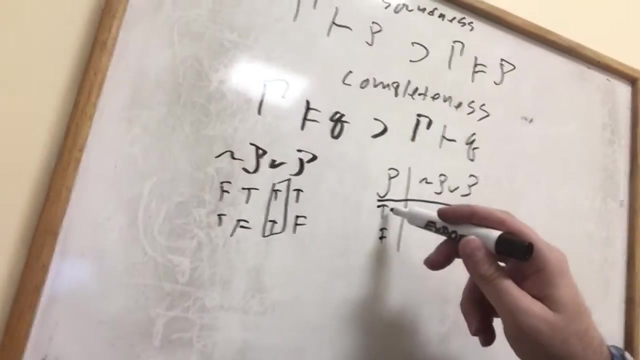 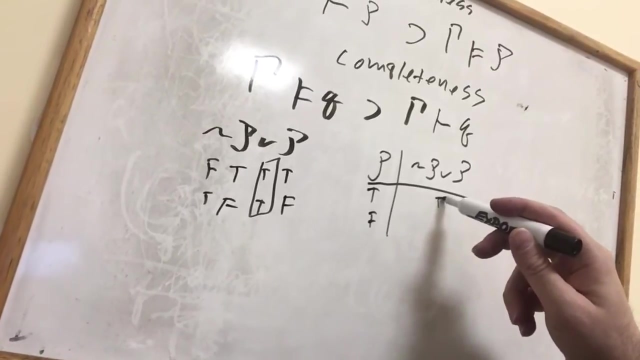 a truth table. so let's look at P and also tilde P, wedge P and there's a point. Okay, so that's what we've done right here, but I'm just kind of making it explicit for us to focus on it. So P can have these two values: it's either true or it's false, and we know what happens when P is true. then the whole sentence comes out to be true. 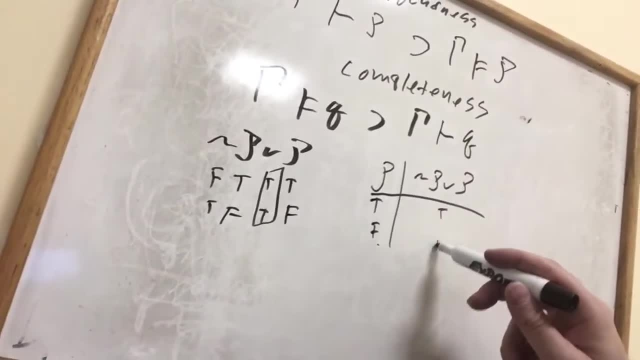 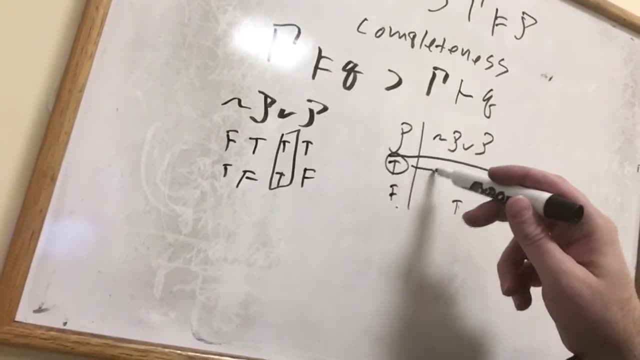 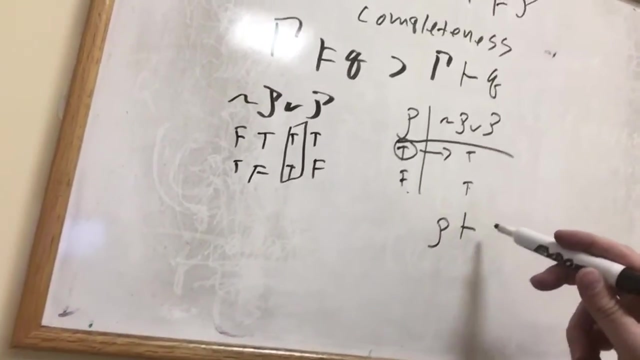 And if P is false, then that makes tilde P true, and so the whole sentence comes out to be true, no matter what P is doing. But look at the case where P is true. Well, we can see that what this is telling us is that P all by itself should syntactically entail tilde P, wedge P. 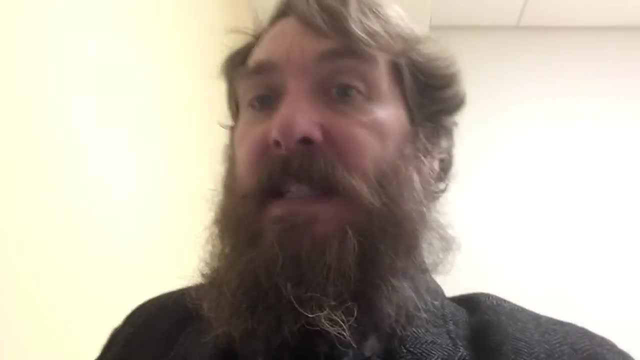 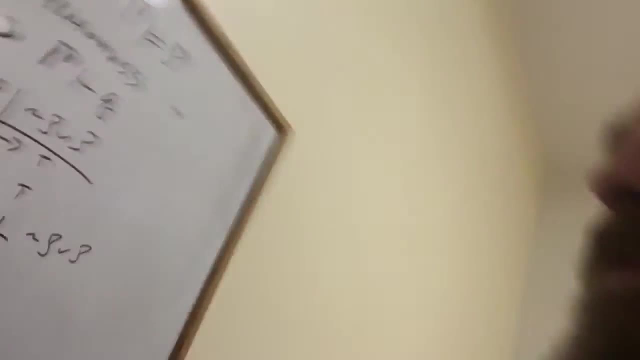 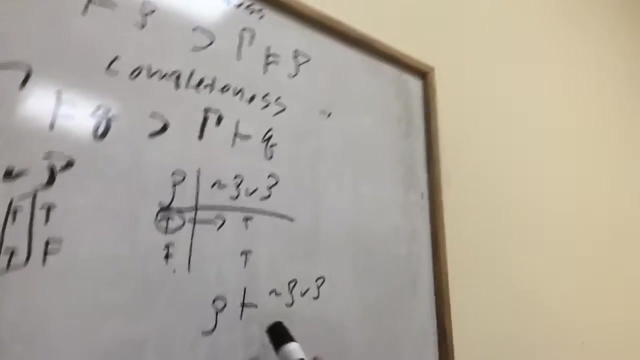 So the truth table, when we examine it, actually tells us straightforwardly, according to our definition of semantic entailment, that there should be a semantic entailment from P to tilde P. So that's interesting. Now look at the case where P is false. 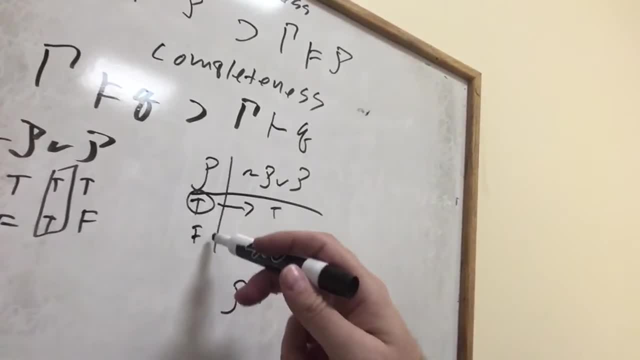 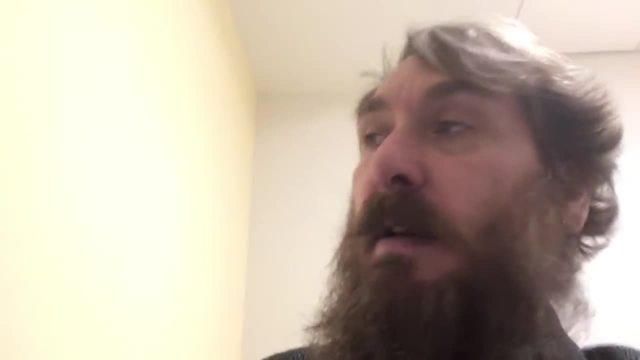 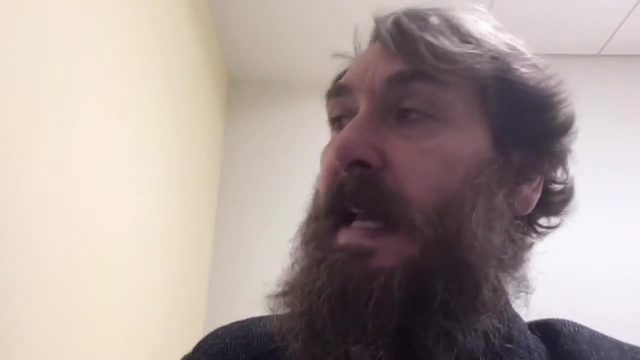 So in this particular case, we can see that that sentence is still true, and so now there's no semantic entailment there, because there's no true and also true. but we can easily turn this into a case where there's a semantic entailment. 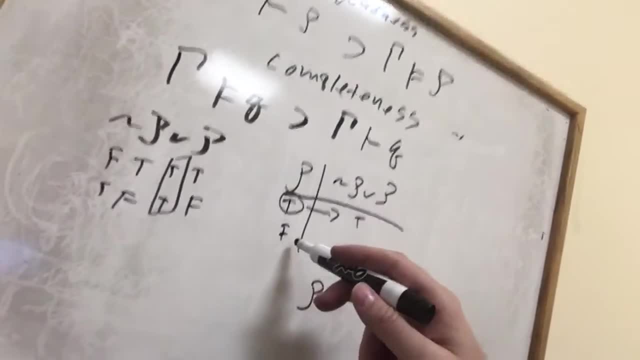 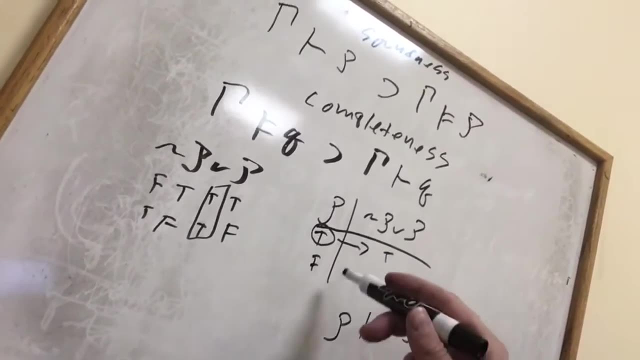 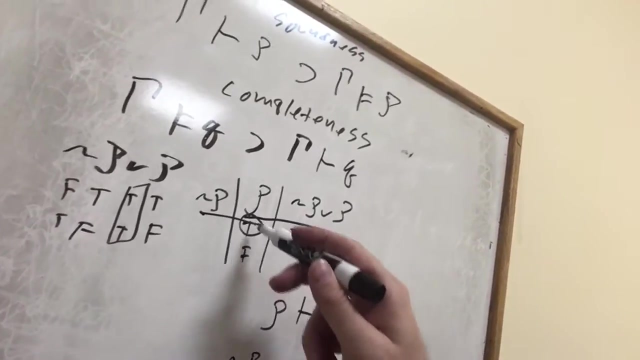 because really, according to our definition of negation, if P is true, then we can easily turn this into a case where there's a semantic entailment. but if P is false, then tilde P has to be true. And so if we looked at tilde P- the truth table for it- then it's the reverse of this, so it's false and true. 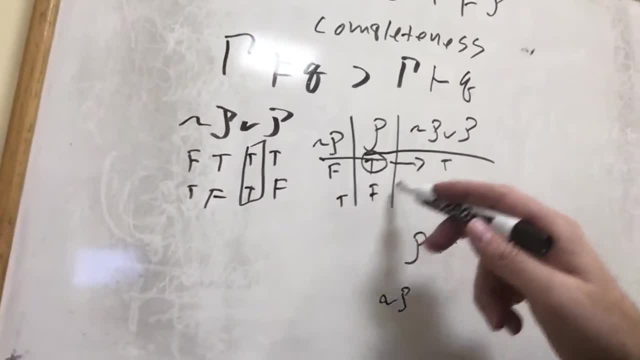 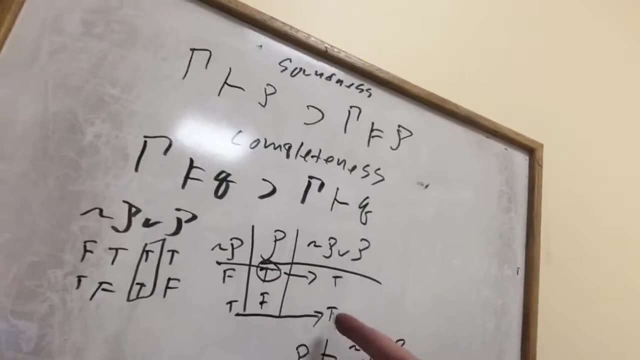 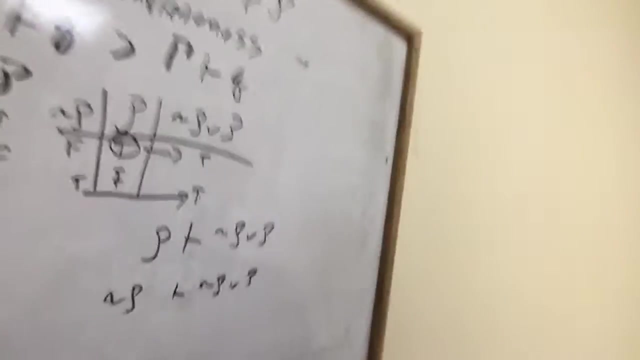 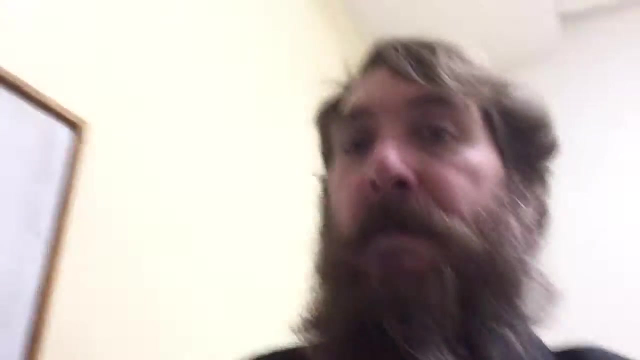 and we can see from this that when tilde P is true, there's a syntactic entailment- excuse me, a semantic entailment. We can see that there's a semantic entailment from tilde P to this thing over here, And so what this is kind of showing to us is that, whether P is true or not, there should be a syntactic entailment to tilde P, wedge P. 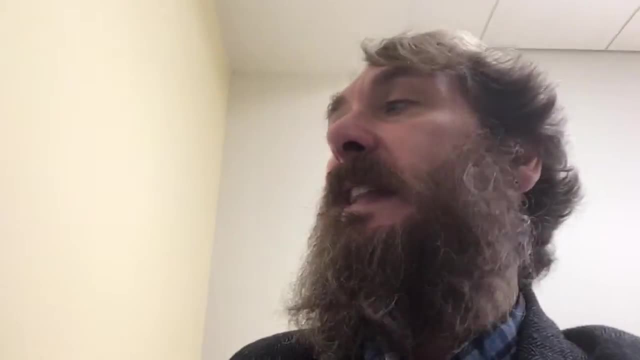 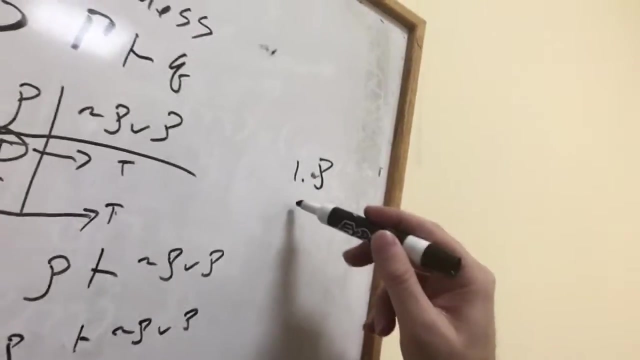 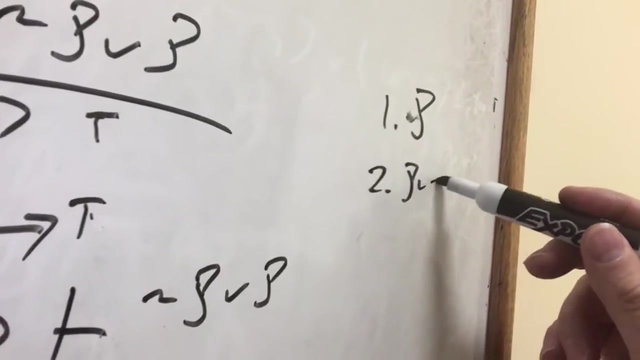 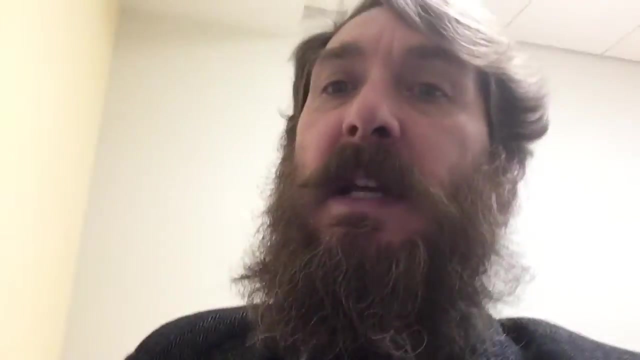 And in fact we can kind of see pretty easily that there is. So if we start from the premise that P, we can use the addition rule. So if we start from the premise that P, we can use the addition rule. And so, starting from P, there is a proof of P wedge tilde P. 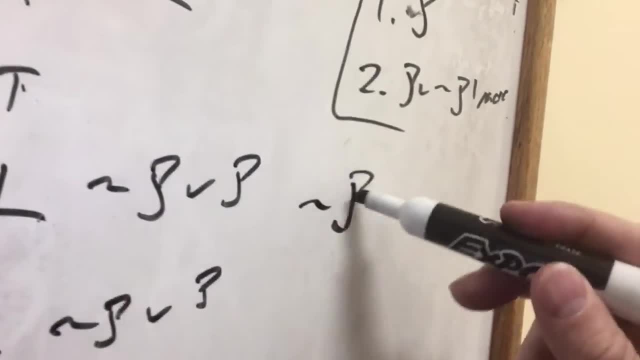 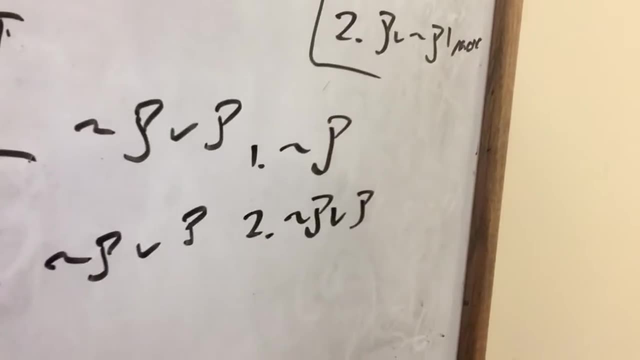 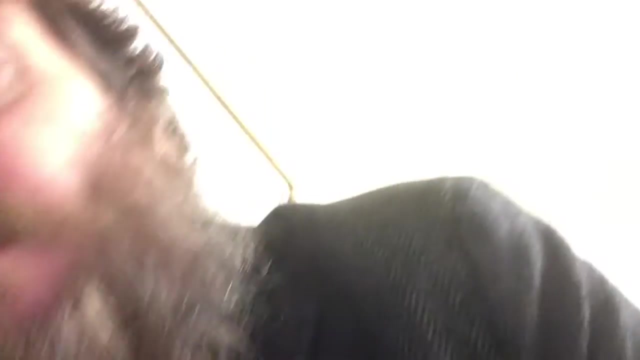 Now, if we start from tilde P, we see there's also a syntactic entailment, because we get tilde P, wedge P And so either one of those that we start with. we can see that there is. sorry, dropped my pen here. 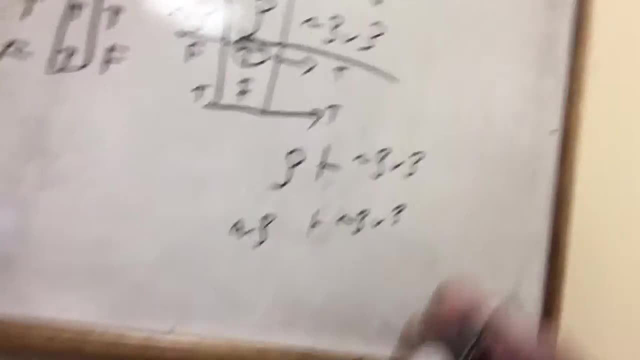 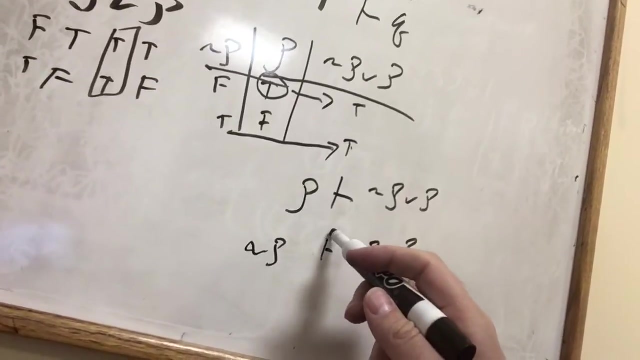 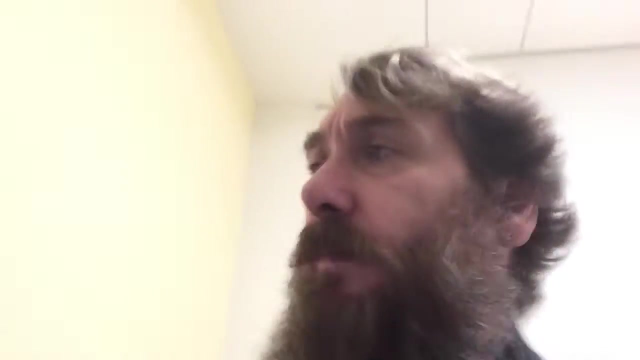 Either one. we start with Either P or tilde P, we can see that there is a syntactic entailment straightforwardly to the conclusion here, And in fact that's enough already for us to kind of see that if this is the case, 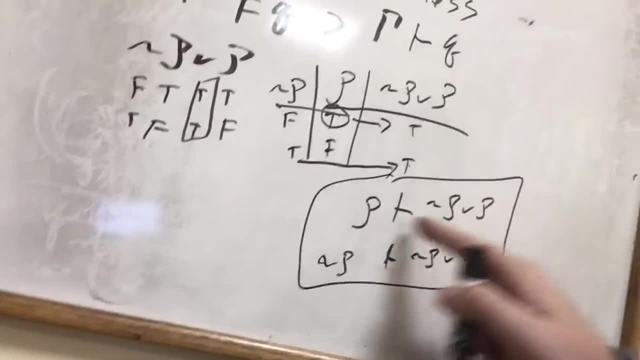 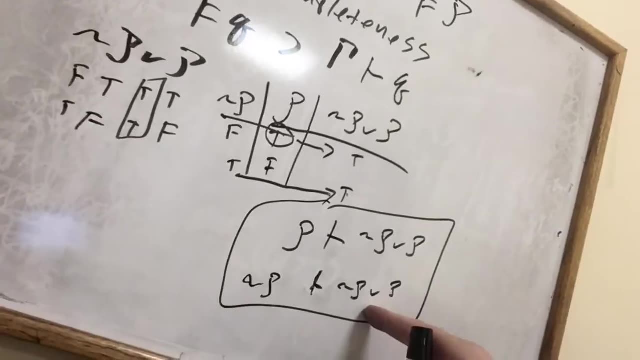 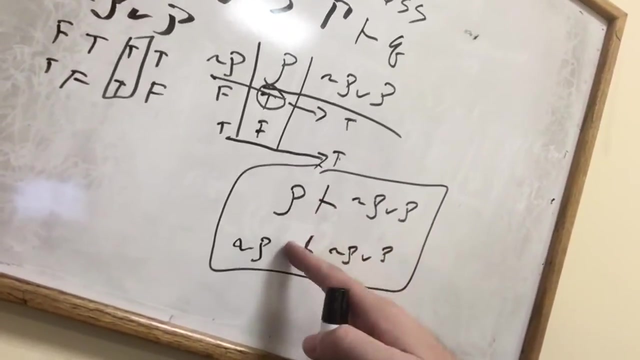 if this is the case- that whether P is true, you get an entailment syntactically, Or if P is false, you can produce tilde P, horseshoe P. What that looks like is that this derivation doesn't in any way depend on P. 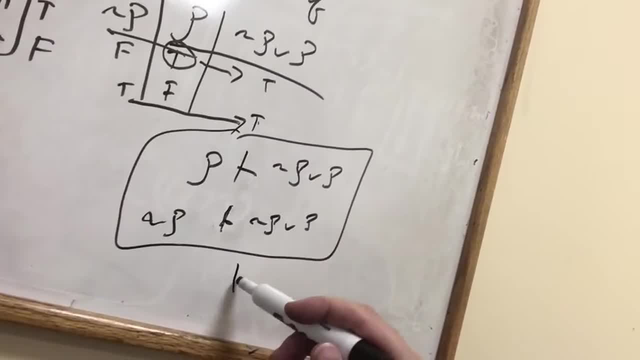 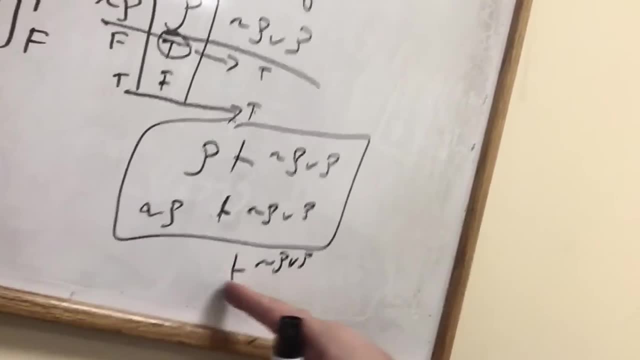 And so it looks like what this is telling us is that, well, it should just be a straightforward syntactic entailment, that tilde P, wedge P, that that should be something that we could produce with no premises at all. And in fact we know. 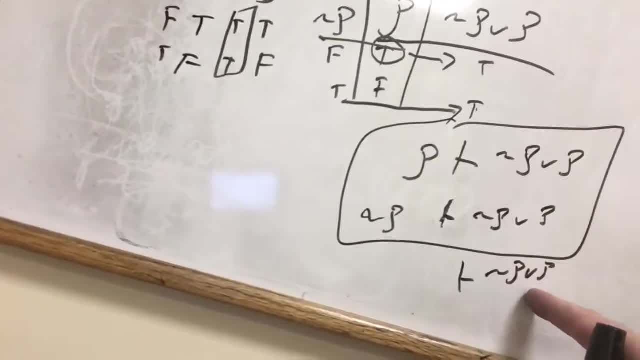 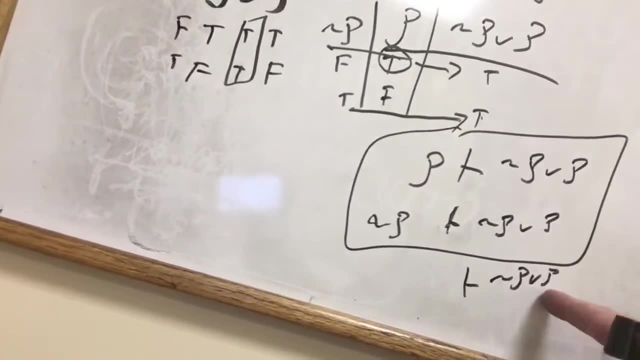 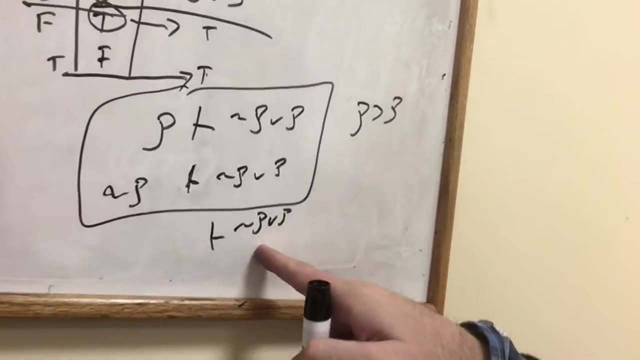 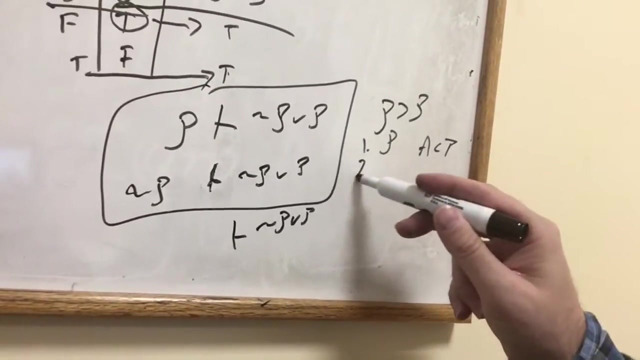 We know that that's something that we could produce with no premises at all. So if we wanted to think about this in terms of a conditional statement, then we know what that really says is that P horseshoe, P by material implication. So what that shows us is that we could start by assuming P for conditional proof. 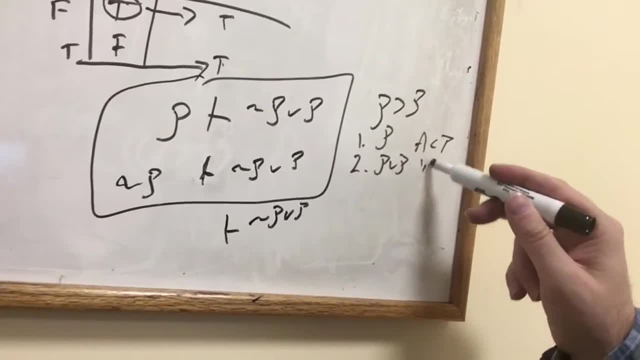 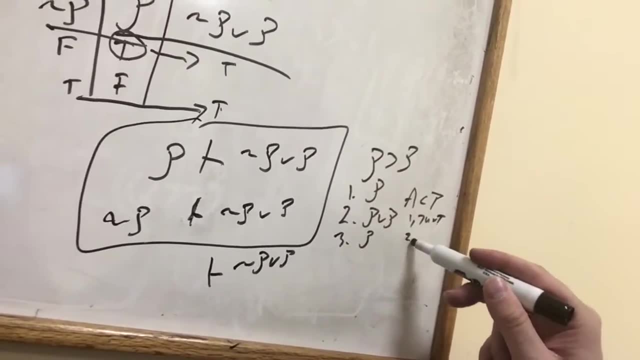 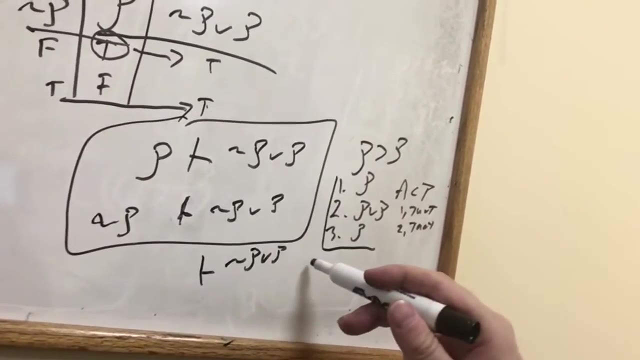 Use the tautology rule, which is annoying, But our system requires that we do that, And then you could use the tautology rule again. You started off assuming P, You ended up producing P, And so you can conclude from that, by conditional proof, that P horseshoes P. 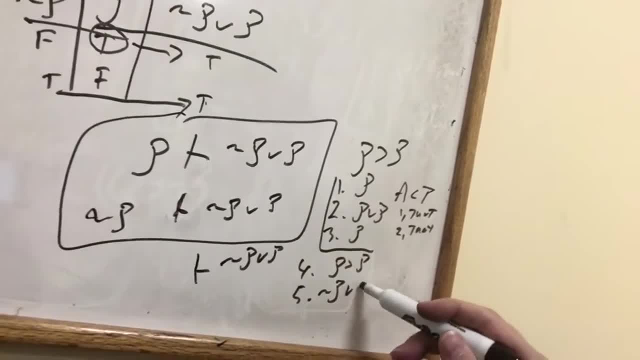 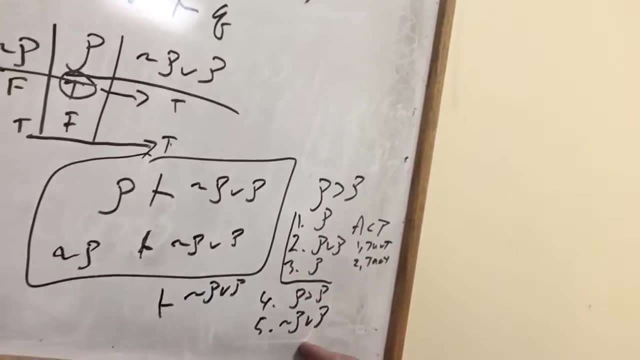 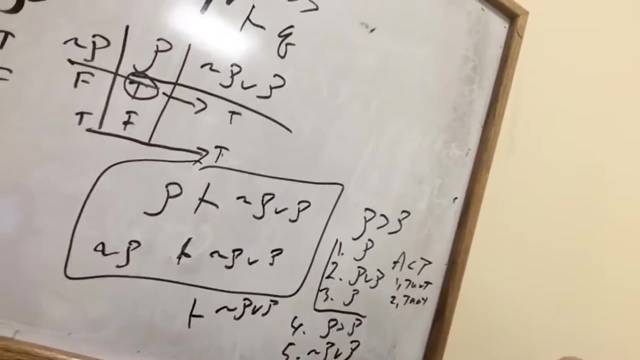 And you can conclude from that, by implication, that tilde P, wedge P. And so you can see that there is a proof with no premises Which the conclusion of which is: tilde P, wedge P. So now we haven't gone through this in all of the details that we wanted to. 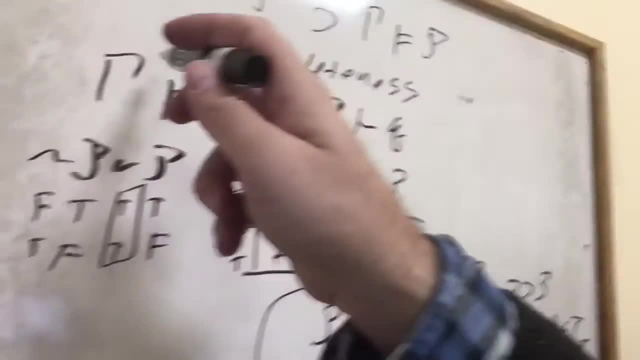 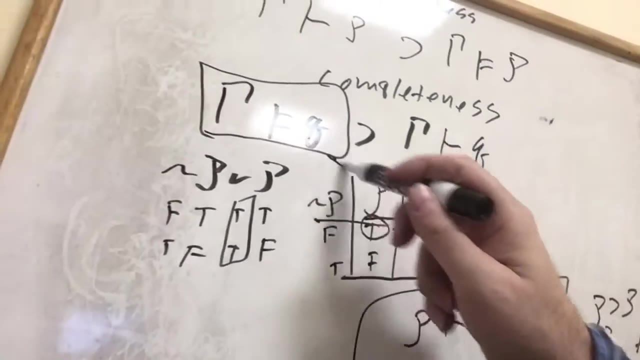 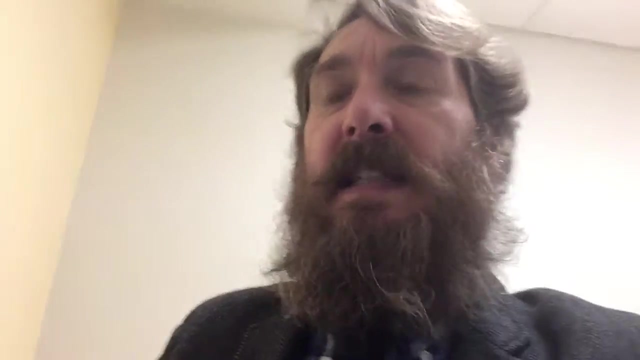 But look, it looks like what we just assumed show was that if you start off assuming that the thing is a tautology, then you will be able to show that there is a proof of that thing, And so it looks like what we've been able to show is that the system is complete. 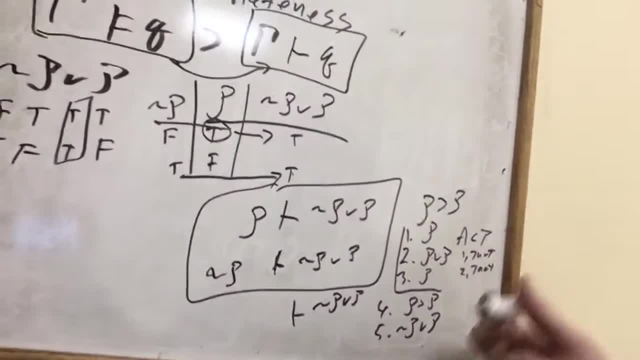 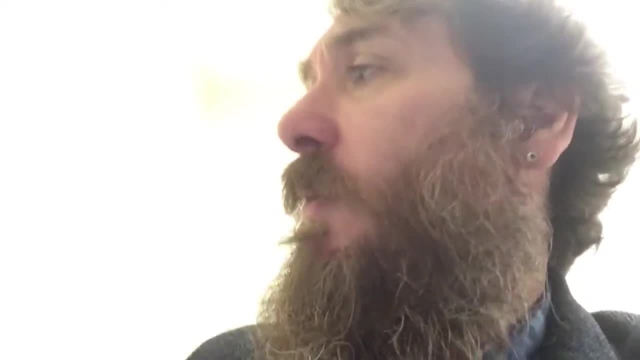 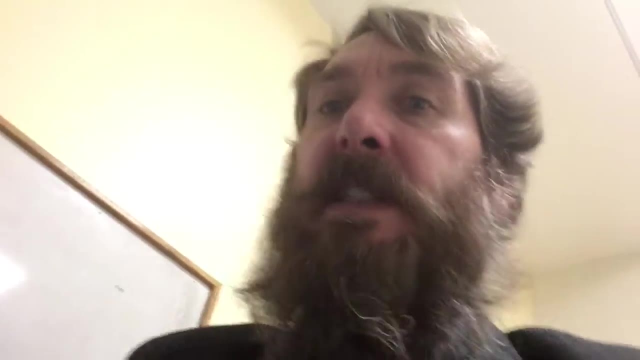 Now, to really be able to rigorously prove this would require some extra work And we would need something called the deduction theorem. And of course we don't really want to delve too strongly into that kind of stuff, But in case there is some interest in that, the deduction theorem roughly says the following thing: 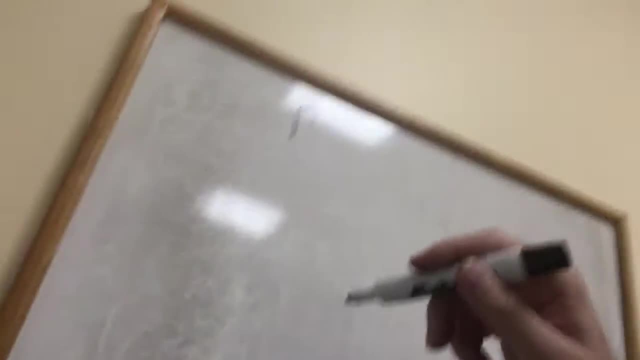 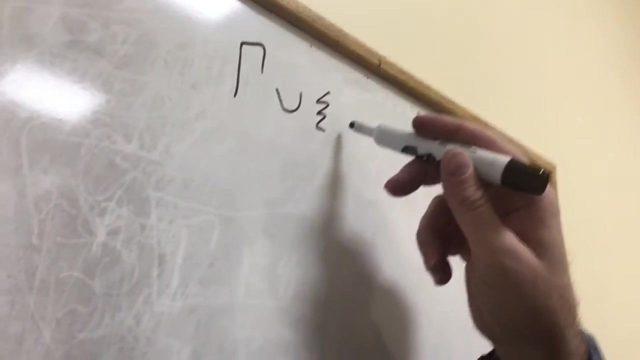 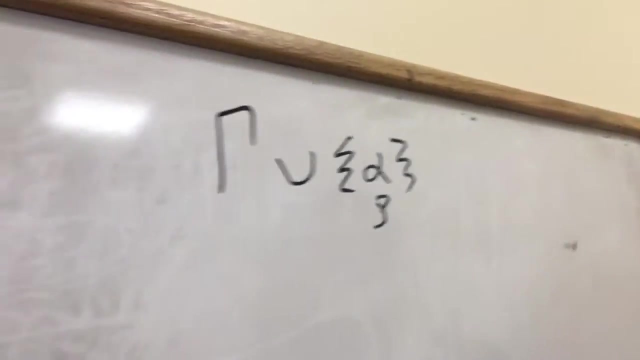 It says that if there is an entailment from a set of sentences, gamma, if there is an entailment from that and the union of that with some proposition, normally designated as alpha, but in our system we would call it P, probably because of the way that the notation of our book works. 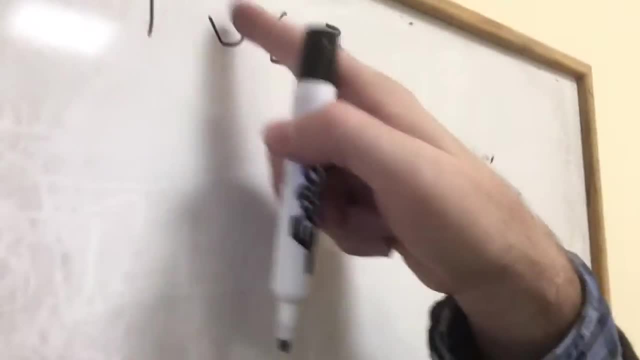 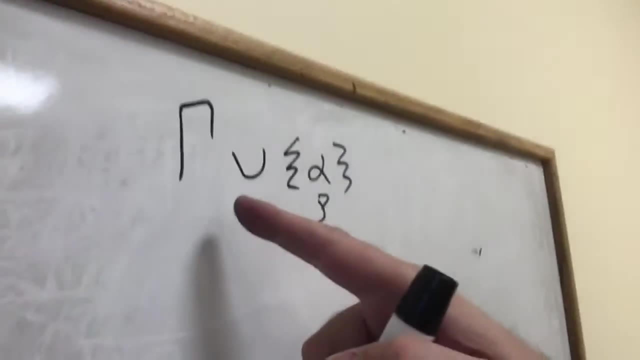 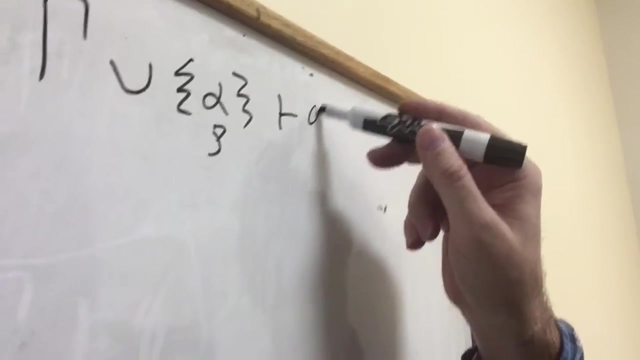 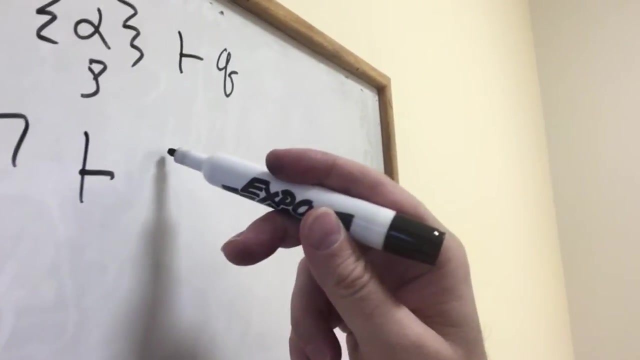 So if the union, which basically may mean these two things together. So this is the language of set notation, but don't worry about that. So what this is telling us is that if there is an entailment from these things to some proposition, then the set of sentences over here all by itself entails syntactically that P, horseshoe, Q. 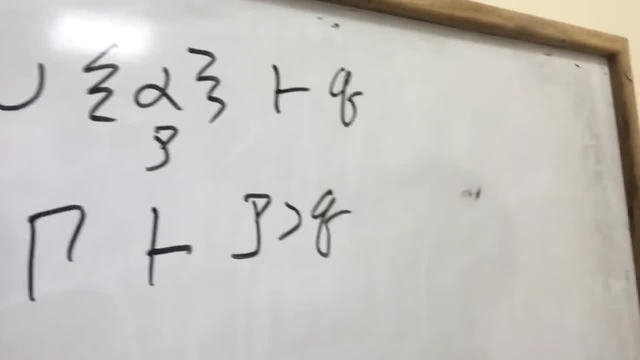 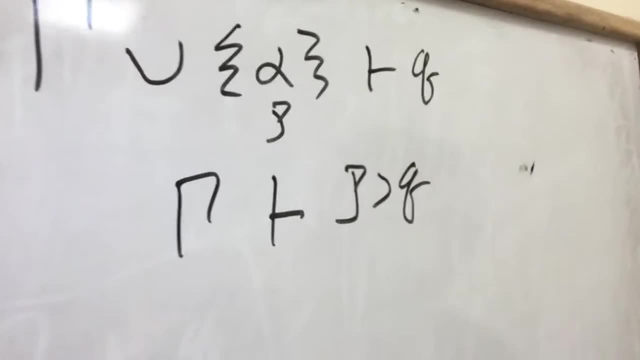 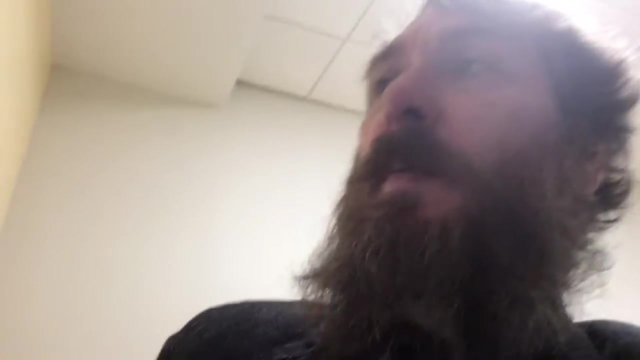 So the deduction theorem tells you that you can. if you know this, then you can always take one of the premises of your argument and show that there's a conditional statement which could have been proved without that. So why is that interesting? Well, because notice that what we had just shown a second ago was that P entails. 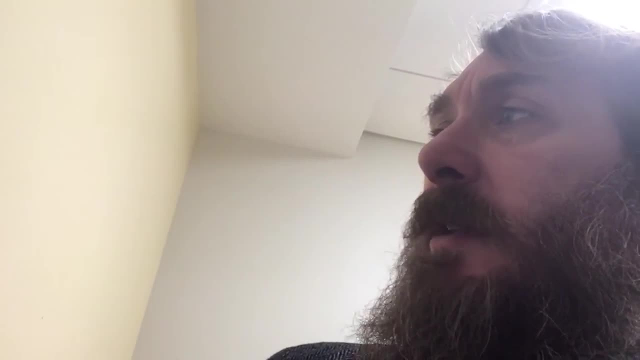 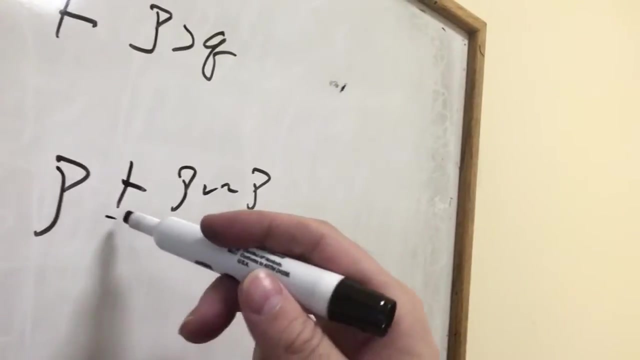 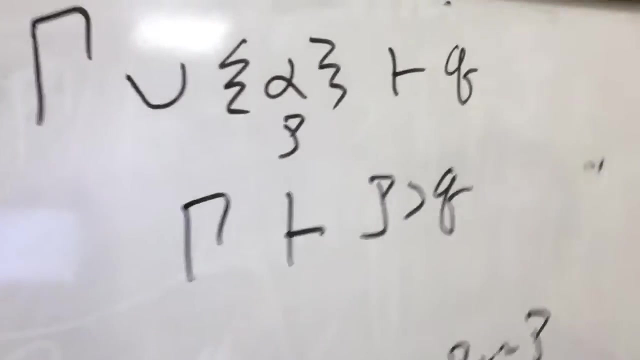 syntactically that either P wedge tilde P. Okay, so here we have a syntactic entailment from P to P wedge tilde P, and we've seen how we could produce that. And so we look at the deduction theorem and it looks like what we have here. 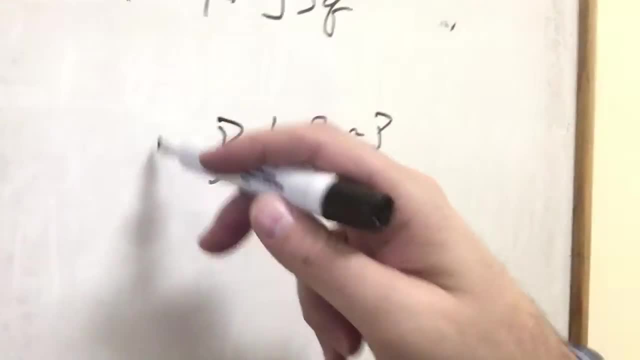 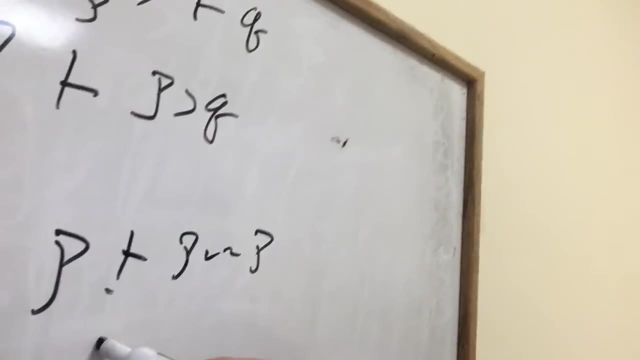 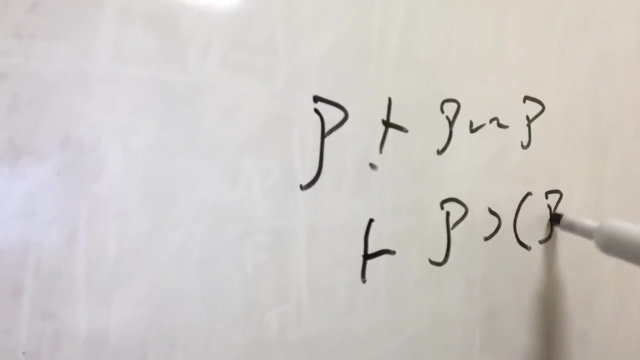 is the claim that there's the set of sentences, That there's the set of gamma, which is the empty set along with P, entails that, And so the deduction theorem says that we should be able to take P and move it over here and get a syntactic entailment from P to the horseshoe of P. wedge, tilde P. 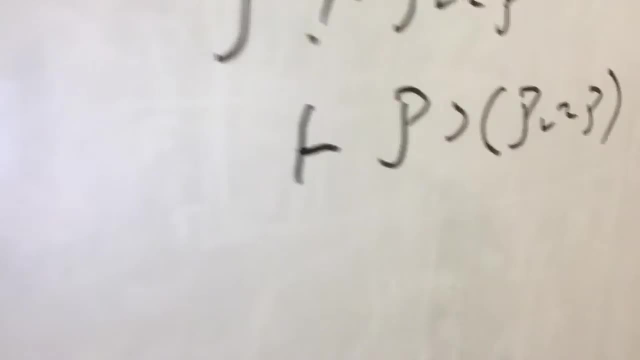 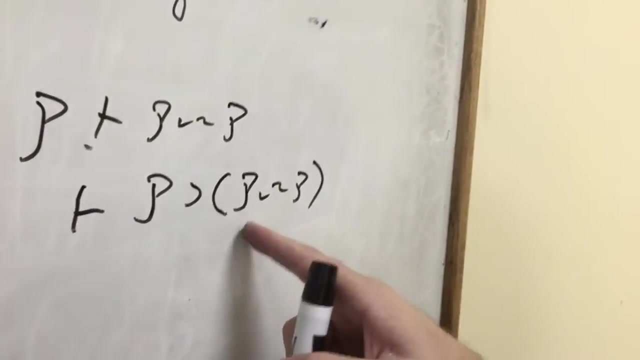 So that there should be a proof of that. And that's good, because then we could see by using a little bit of logic on P horseshoe, P wedge P, that that's really just largely equivalent to saying there's a proof of P wedge P. 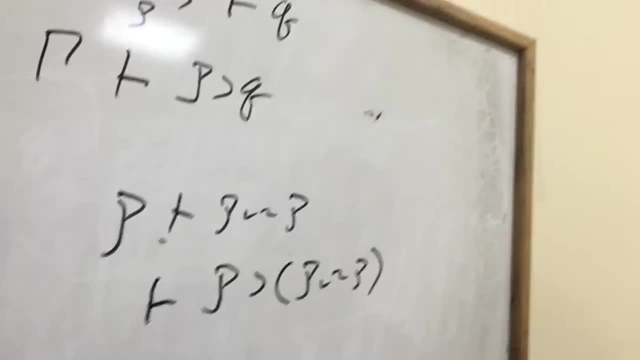 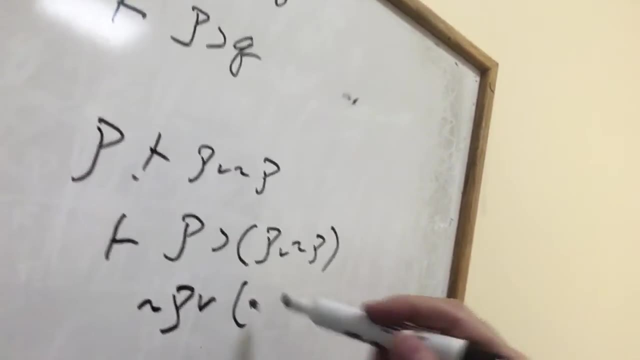 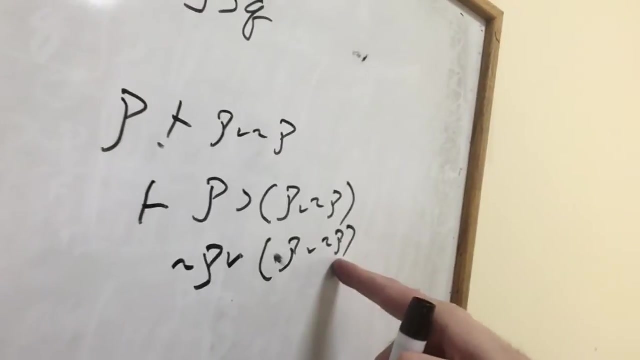 So we could do that a couple ways, but one way of doing it is as follows: So we use implication, we get tilde P, wedge P, excuse me, P wedge, tilde P. Okay, and now you can see here that if you use com, you're going to get tilde P, wedge, tilde P, wedge P. 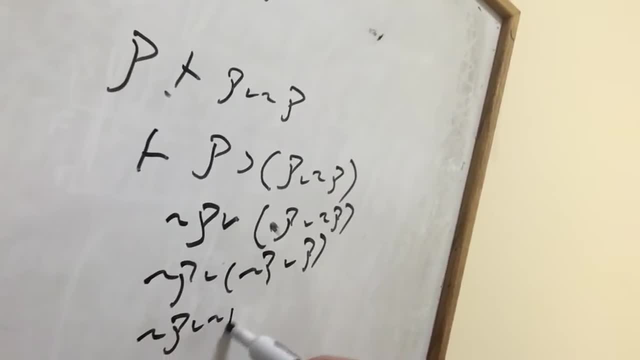 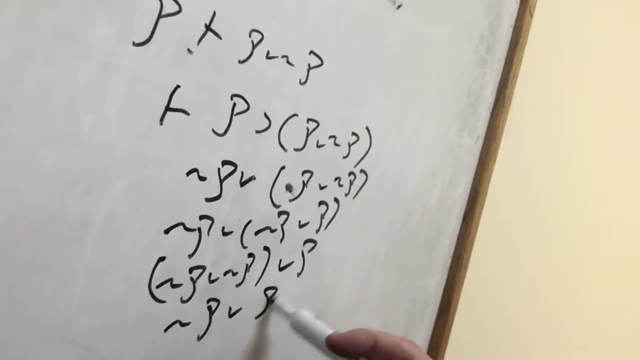 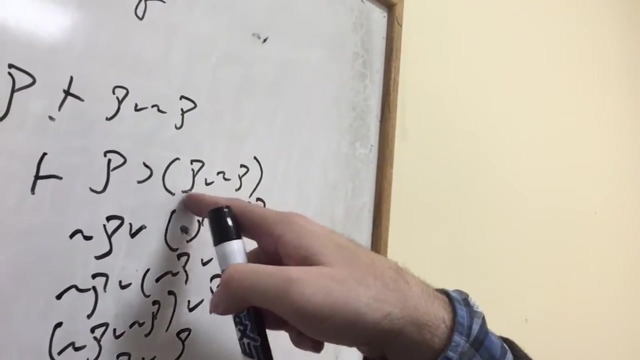 And then use associativity- Tilde P, wedge, tilde P, wedge P, And then, using the tautology rule, gives you just tilde P, wedge P. And so you can see that by the statement that P horseshoes the disjunction of P or tilde P. 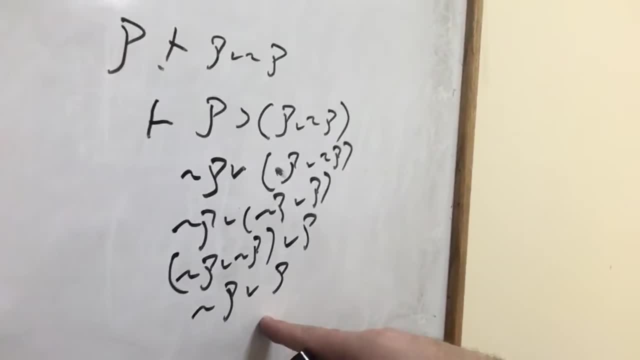 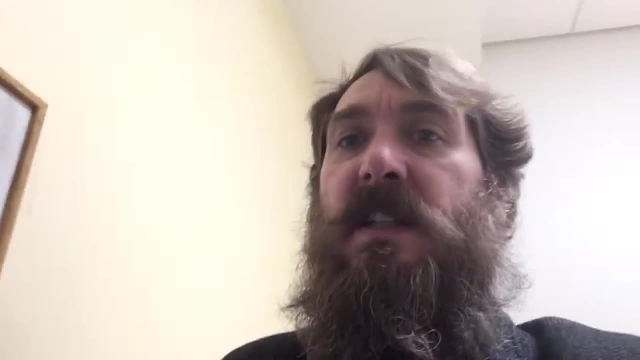 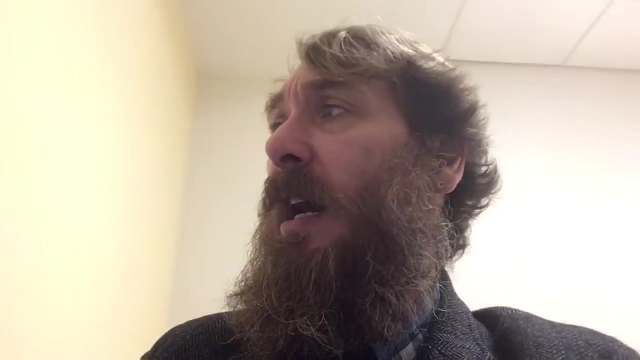 is just the same as saying that tilde P, wedge P, And so saying that there's a proof of this is simply saying that there's a proof of the original thing, And so the deduction theorem here allows us to connect the statements that we were saying previously with what we were just doing. 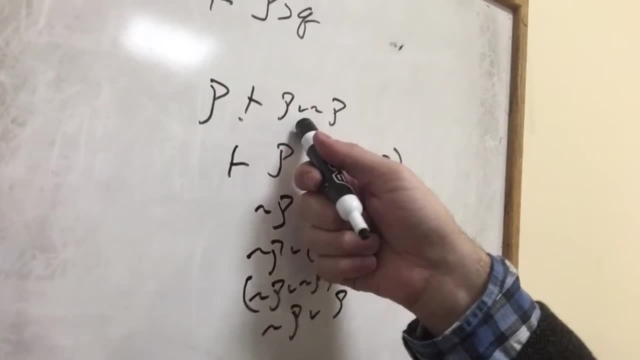 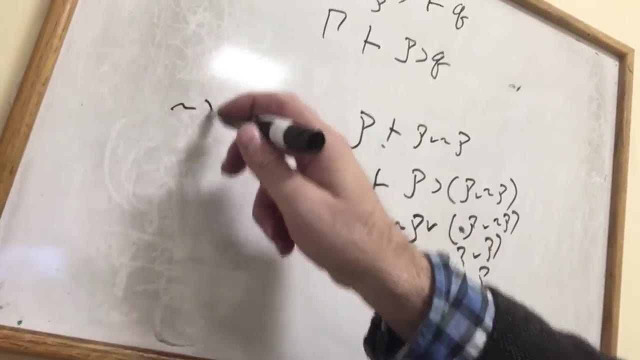 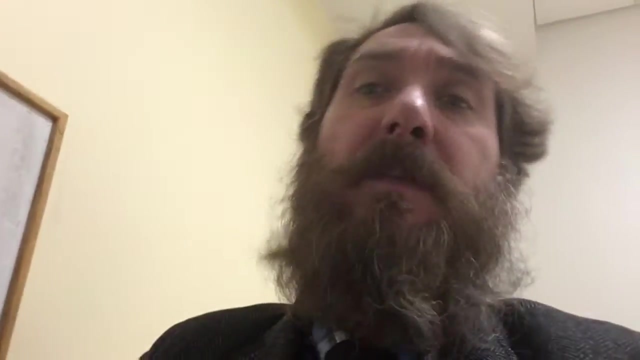 Because what we have just shown is that if P entails that, then there's just an entailment from nothing to that. And of course we could do the same thing by showing that if tilde P syntactically entails- or I guess you know to be a stickler- we should say proves, or something like that. 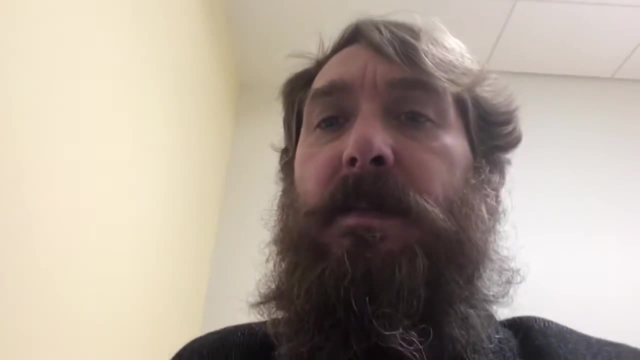 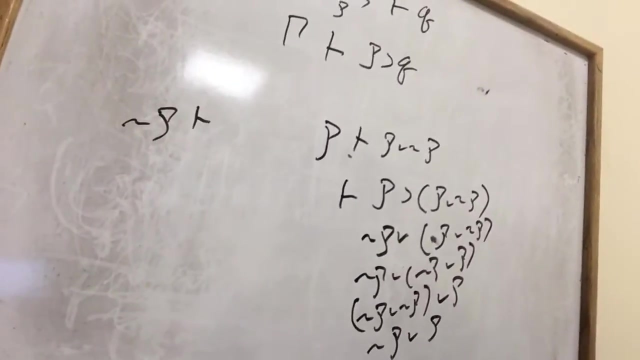 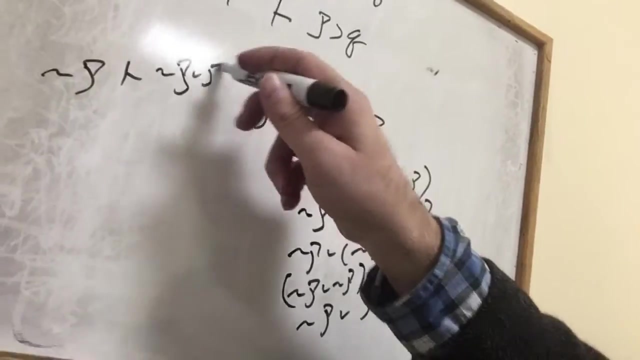 But you know, entails is kind of a semantic notion, So maybe there'll be some people who object to that, But for us, at this beginning level, I don't think it's too terrible to say syntactically entails, Although really we should say tilde P proves that. tilde P, wedge P. 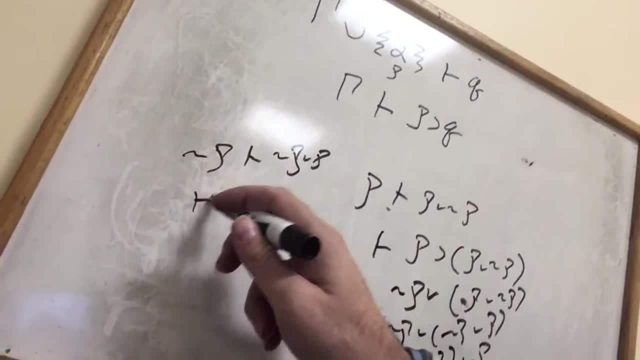 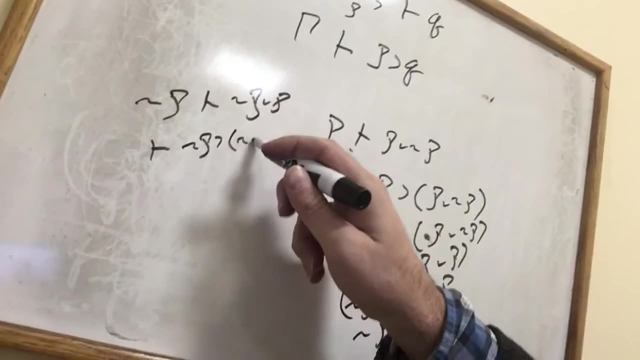 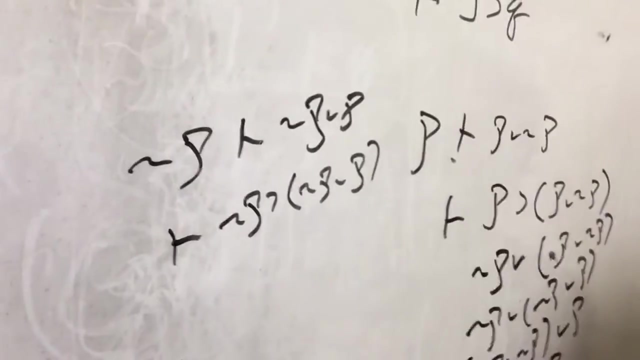 And of course what that shows us is that we should be able, by the deduction theorem, to show that we can prove that tilde P horseshoes, tilde P, wedge P, And I think you can see pretty straightforwardly that this thing right here. 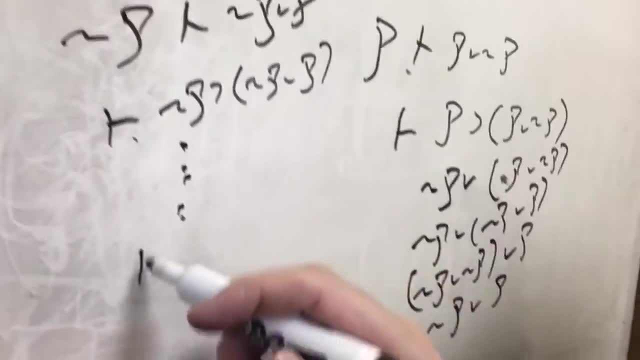 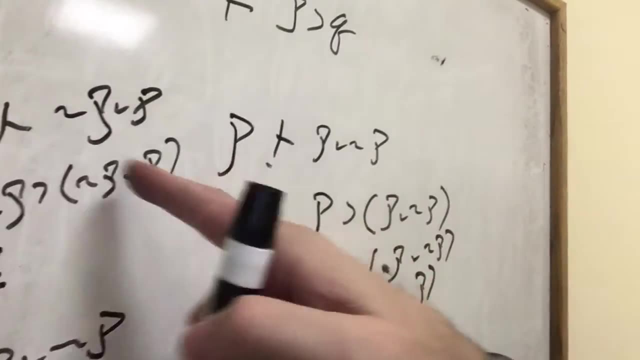 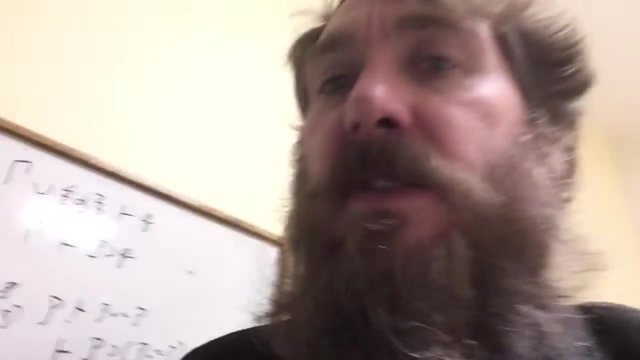 basically by some steps, is just going to show us that we can prove that tilde P, wedge P. So now the two of these together show us that there's always going to be a syntactic entailment. And of course we didn't do this rigorously because we were talking about kind of an example. 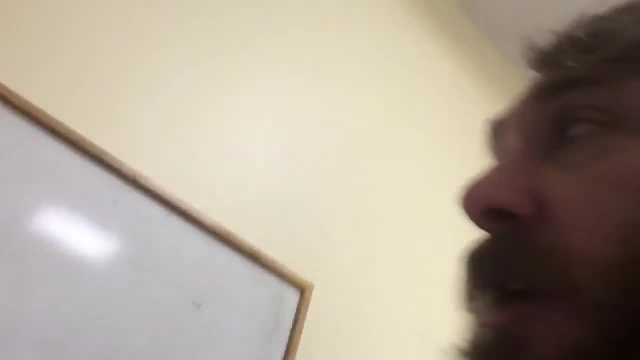 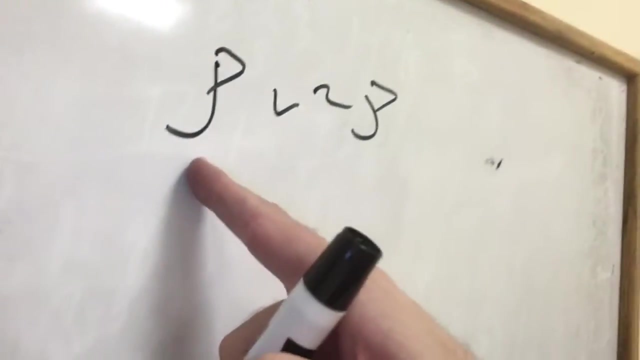 of tautology. So we started off by saying, look, let's take some tautology P wedge tilde P, where at least this is general enough that this could be A wedge tilde A, or it could be A horseshoe B- wedge tilde A, horseshoe B. 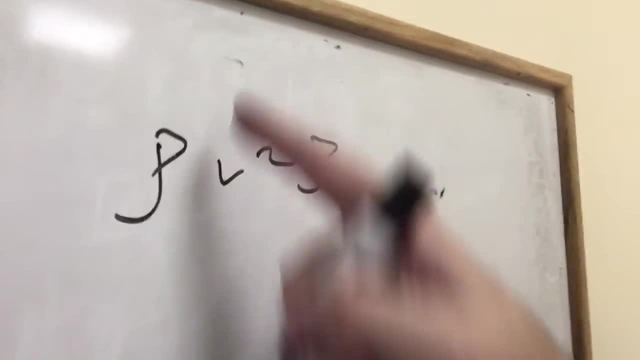 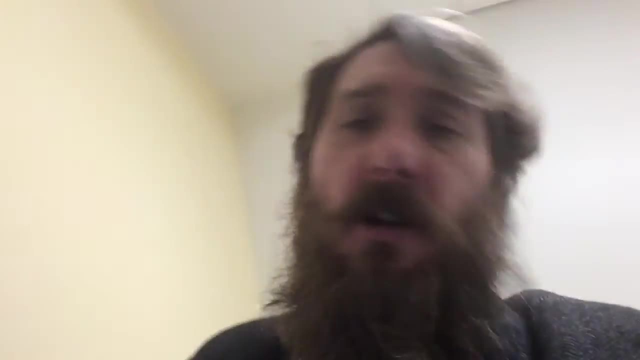 So it could be any of a number of statements, but it still is kind of an example And we haven't. there are all kinds of other tautologies And so we would need to go through all the kinds of different cases showing that we could do this same procedure. 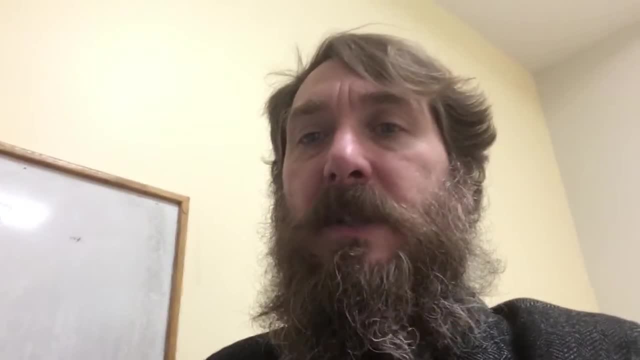 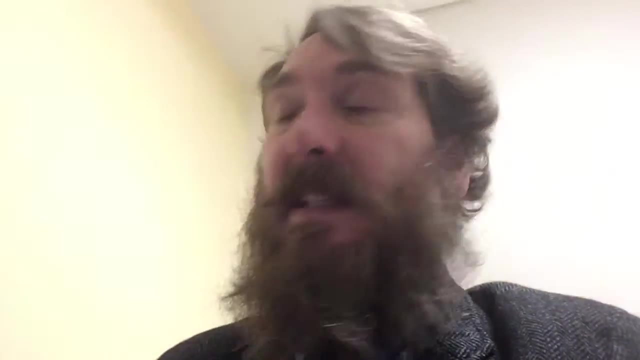 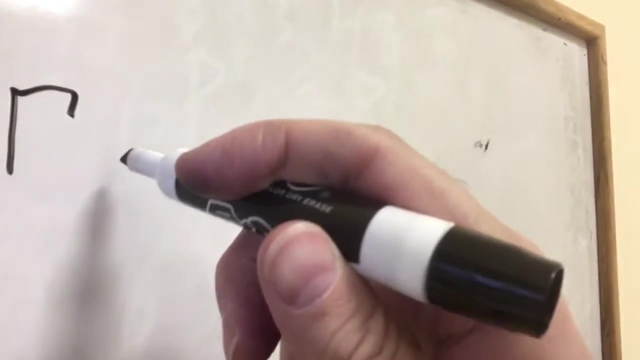 But at least I think you can see from what we have said that the procedure could be done, And so the language that we have at this point, propositional logic, is complete And it's also sound, And so what that means for us is that if we have a set of sentences, 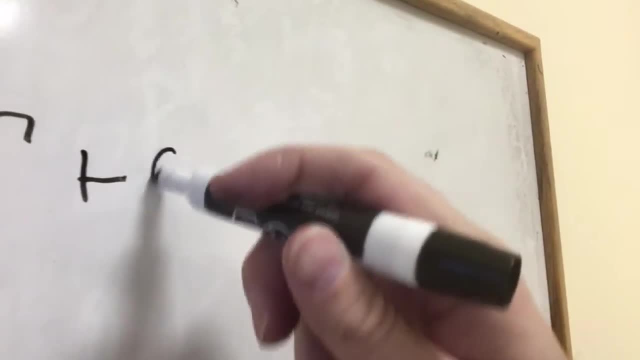 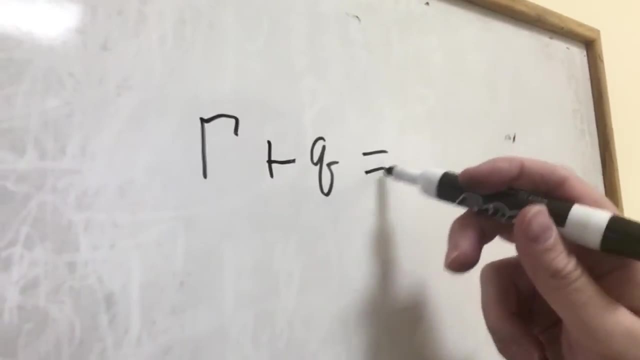 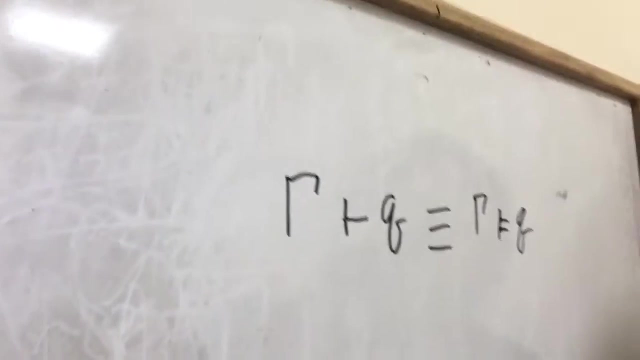 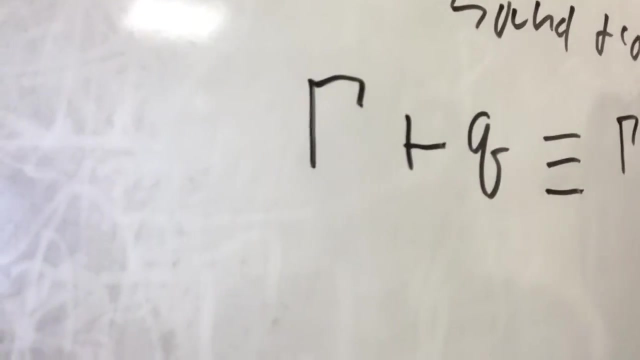 which can prove some other proposition that then we know that that's the case if, and only if, that set of sentences semantically can produce that entailment, And so this tells us that it is sound and complete. So propositional logic is a sound and complete logic, sound and complete language. 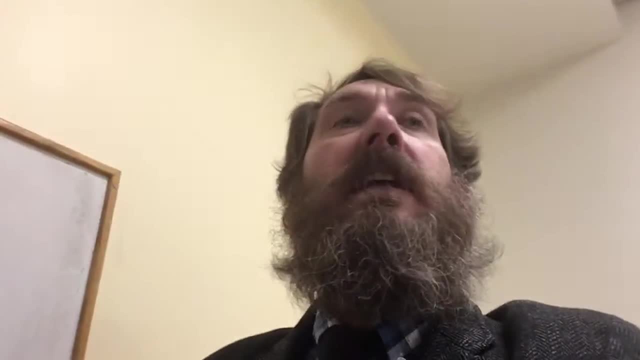 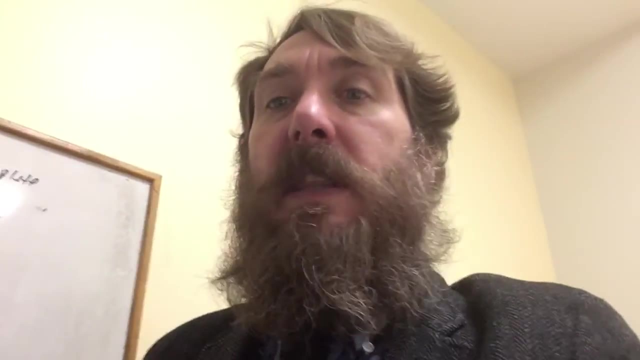 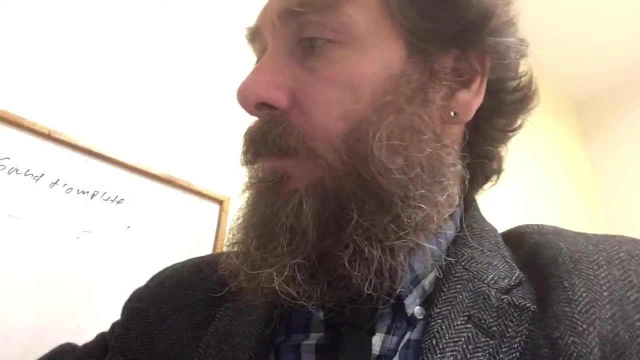 And therefore, what we know is that all and only the things which are true, or valid, or tautological or, depending on how you want to state that, only those things and all of those things can be proved with our system. Now, at that point, we have a structure that we can then take as a core. 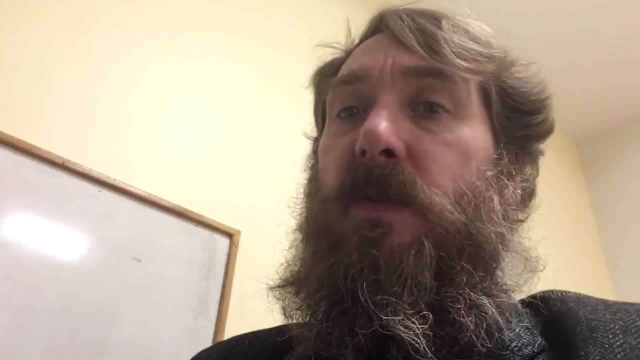 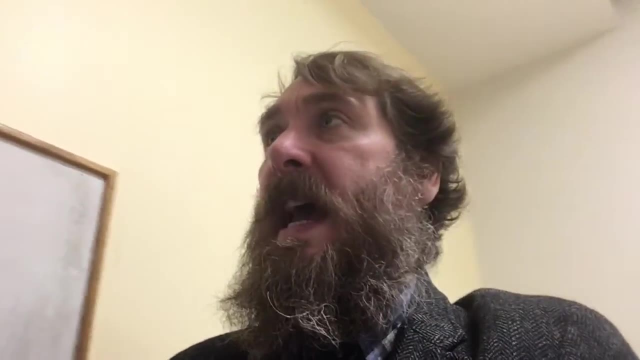 And we can think about trying to add things to it. And so classical logic has as its kind of kernel, at its core it has this kind of notion of propositional logic, truth, functional logic, And then you can take that system, that language. 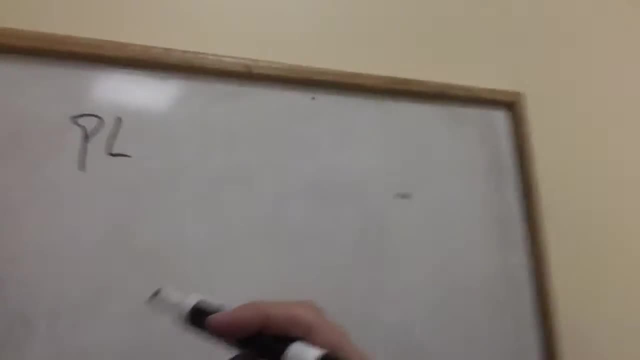 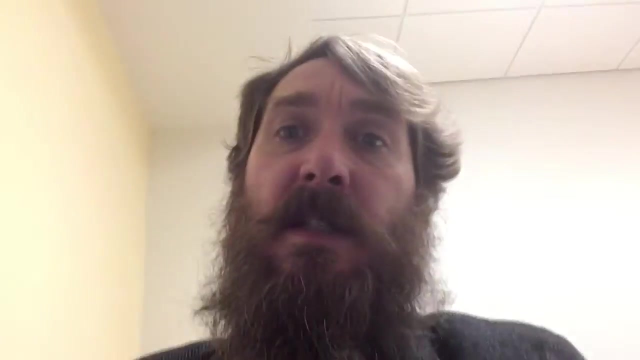 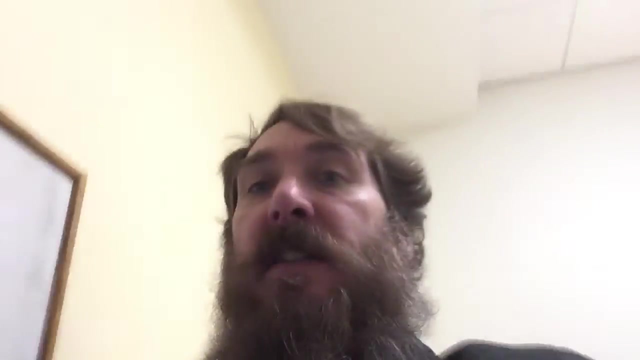 PL, which has all of those elements that we've just been talking about, and then you can add various things to it, And typically the things that you add to it are going to be non-truth functional, And so, for instance, one thing that you could do is to add other kinds of operators.